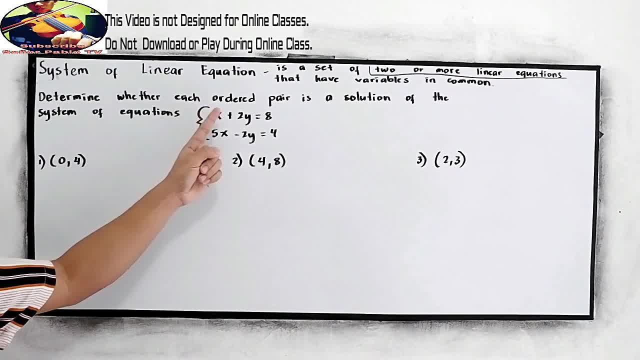 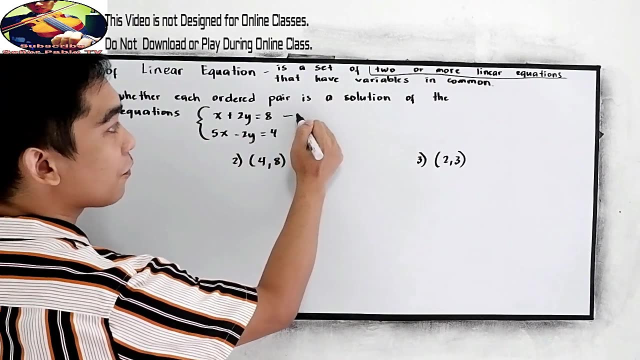 So let's say we have determine whether each other pair is a solution of the system of equations: x plus 2y is equal to 8, and 5x minus 2y is equal to 4.. So we have our first equation here and the second equation. 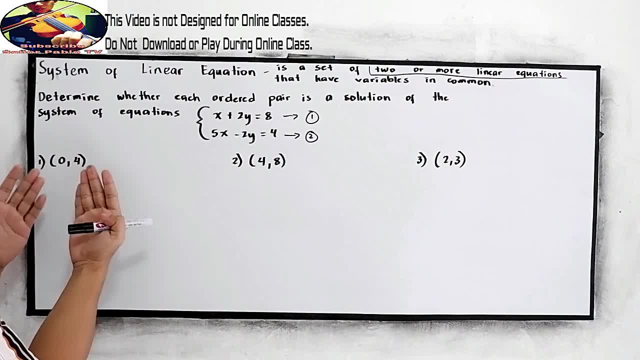 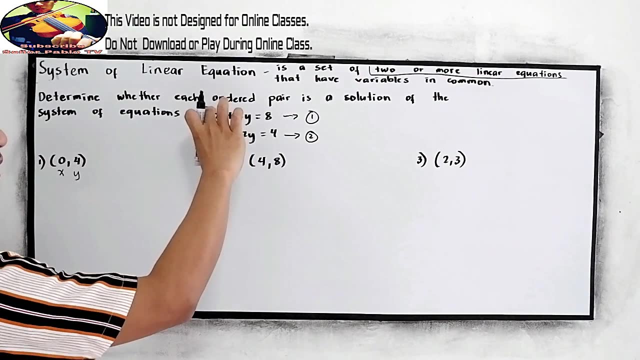 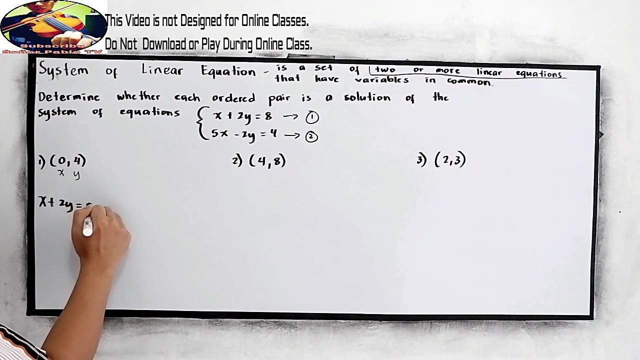 Now since, given the points- let's say 1,, 2 and 3, we're just going to substitute our values for our x and y. So, since this is a point, this is our x and our y. So get the equations. so we have: x plus 2y is equal to 8 and the other one is 5x minus 2y is equal to positive 4.. 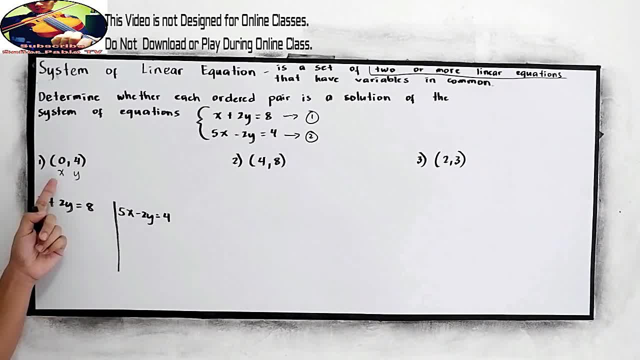 Now in our equation 1, we need to substitute the x and y. So our x is 0. Plus 2 times our y is 4, is equal to 8.. So 0 plus 2 times 4,. so 0 plus 2 times 4,, that is 8, is equal to 8.. 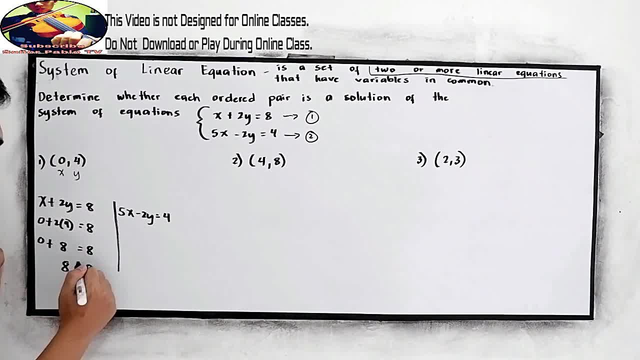 0 plus 8,. this is 8, is equal to 8.. So they are equal. That means 0 is a solution of this. Now let's check our y. 5 times 0 minus 2 times y is 4 is equal to 4.. 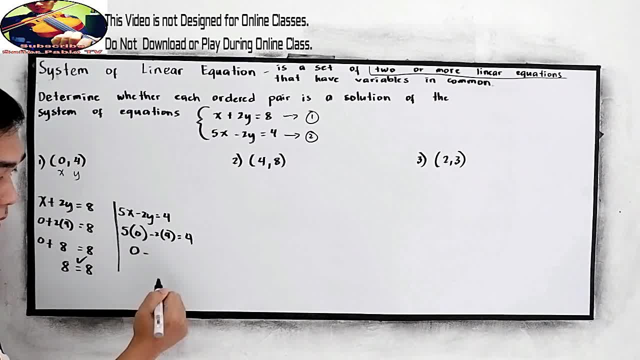 5 times 0, that is 0,. minus negative 2 times 4,, this is 8, is equal to 4.. Negative 8 is not equal to 4.. So this is true, while the other one is false. 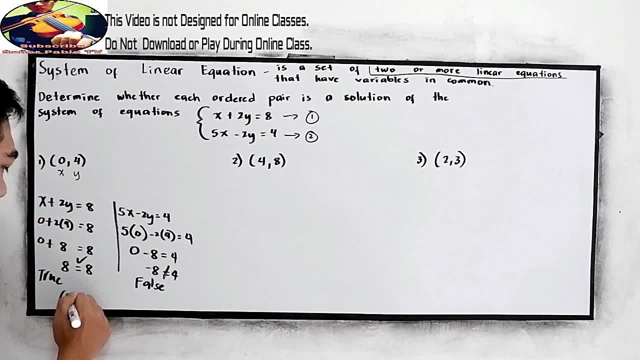 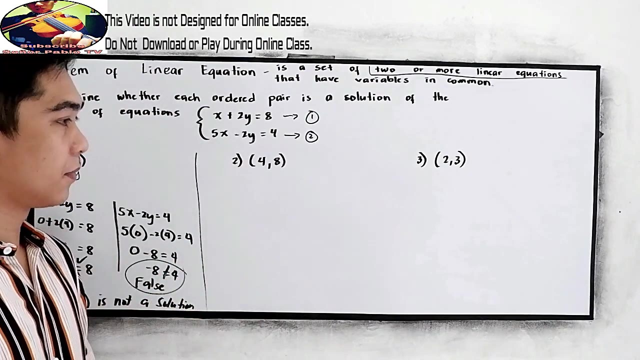 So that means 0,. 4 is not a solution of the system of equation. Why? Because it gives us false answer in our equation number 2.. And now let us proceed in our equation of problem number 2.. And now let us proceed in our problem number 2.. 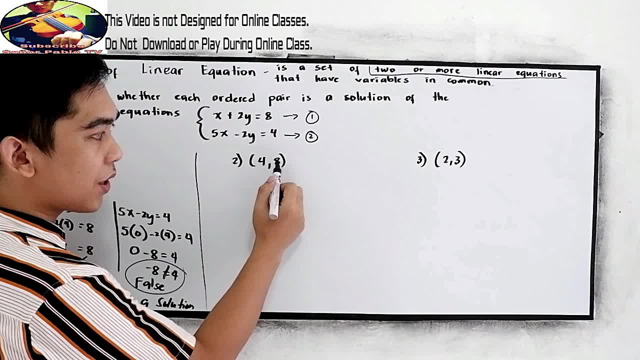 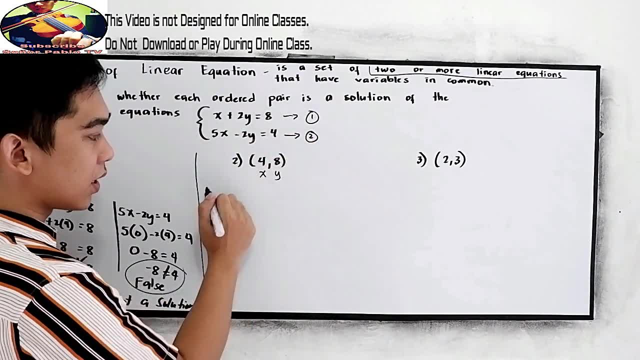 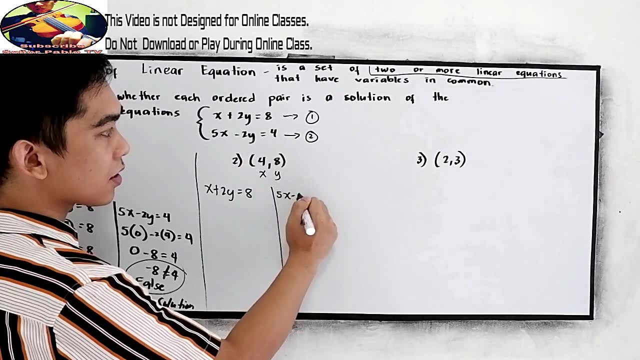 We have a problem. We have a point 4, 8.. So this is our x and this is our y, Copying our equation 1.. So x plus 2y is equal to 8.. And the other one, 5x minus 2y, is equal to 1.. 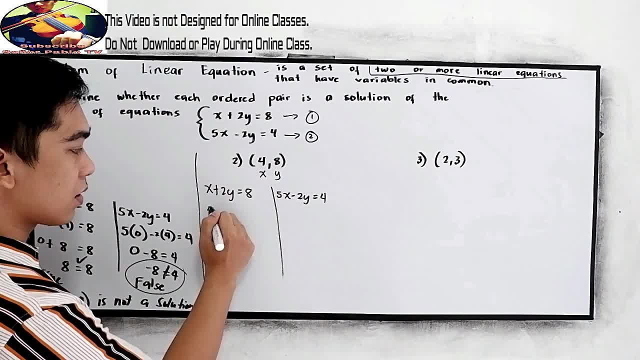 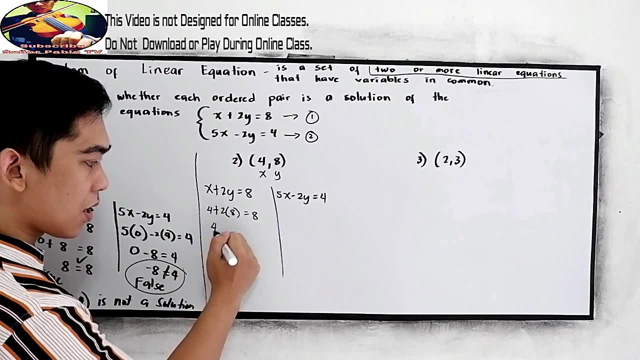 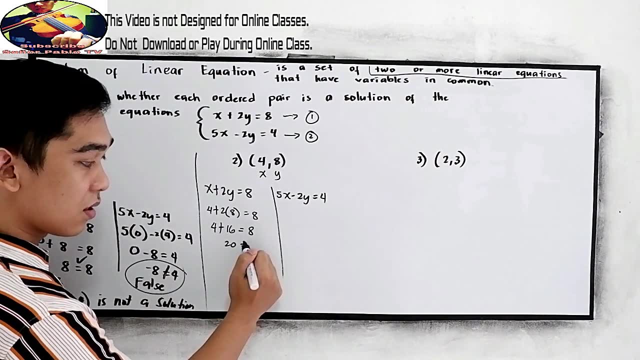 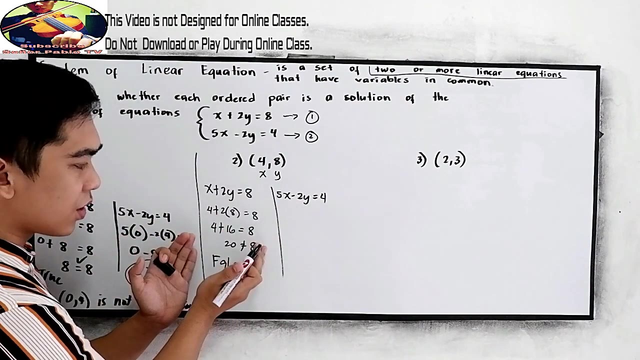 Now substitute: So 4 plus 2 times 8 is equal to 8.. 4 plus 2 times 8 is equal to 16.. So 20 is not equal to 8.. False, So in our first equation it gives us a false answer. 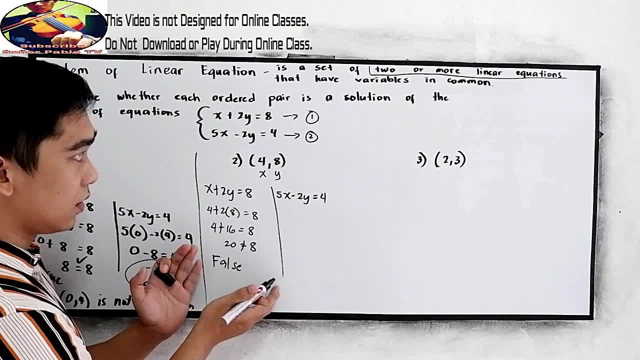 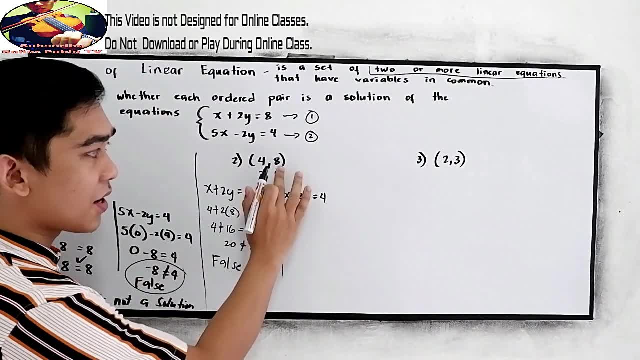 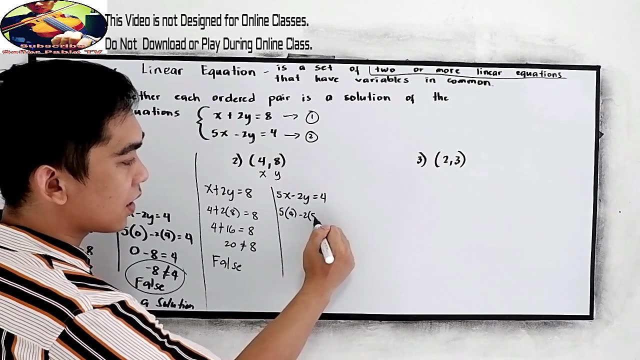 We're going to test for the x and y So automatically. this is not the solution of our system of equations. Now let us check the other equation. So 5 times 4 minus 2 times 8 is equal to 4.. 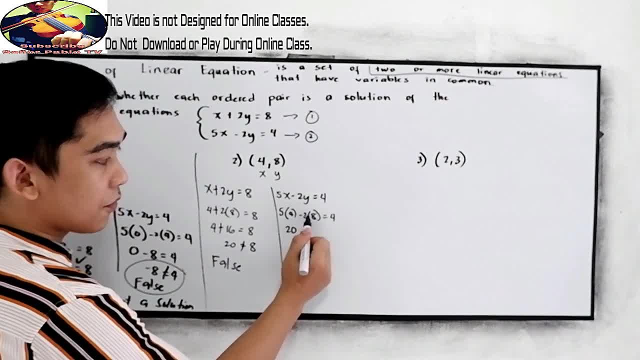 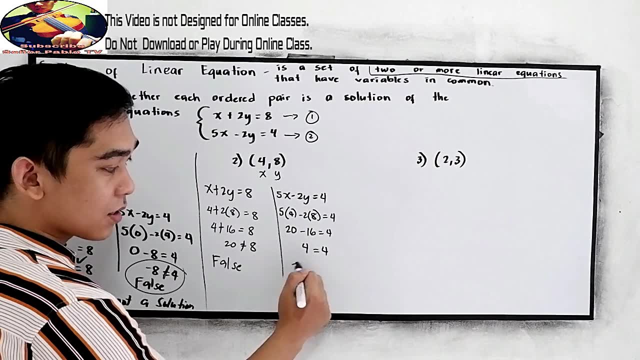 5 times 4 is 20.. Negative: 2 times 8, 16 is equal to 4.. 20 minus 16, 4 is equal to 4.. This is true, Although the other equation gives us a true answer. 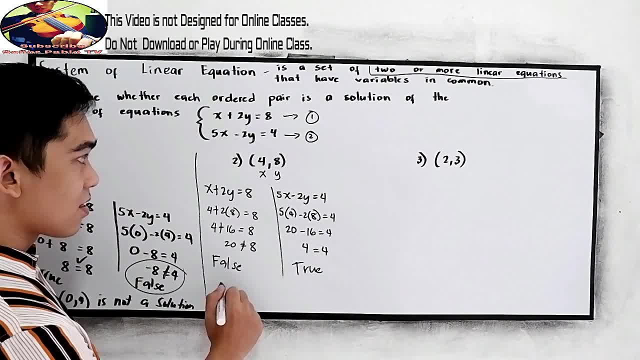 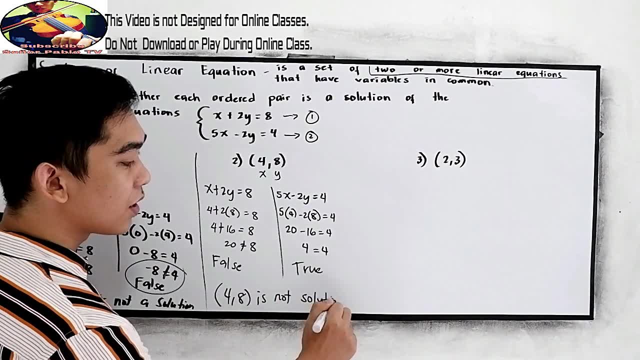 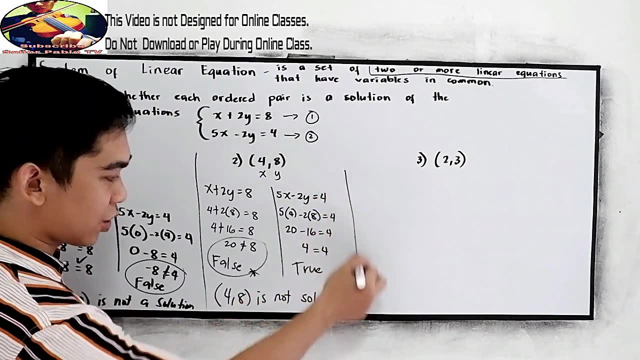 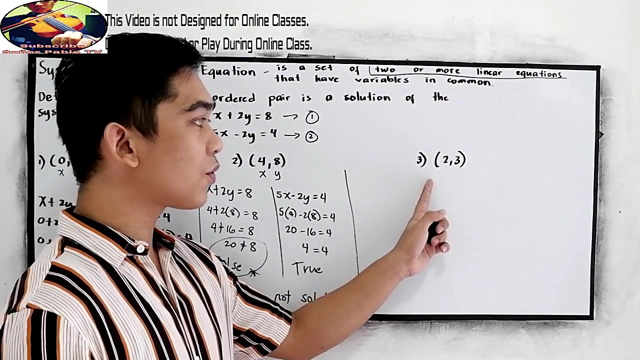 it's still the 4 and 8 is not. This is not a solution of the given system of equations. Why? Because this gives us a false while testing our equation, Just like in our example number 1.. Next, let us try example number 3 or the problem number 3.. 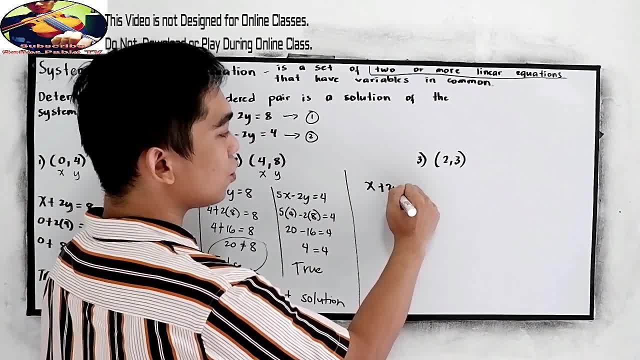 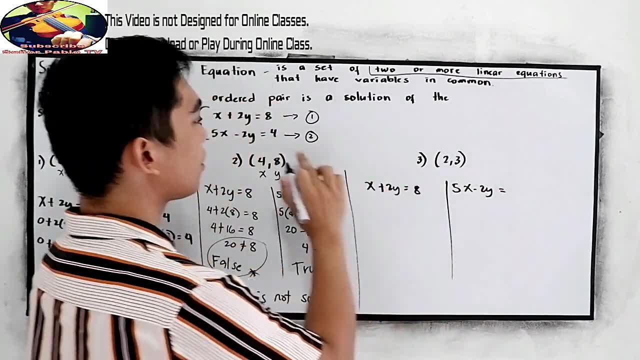 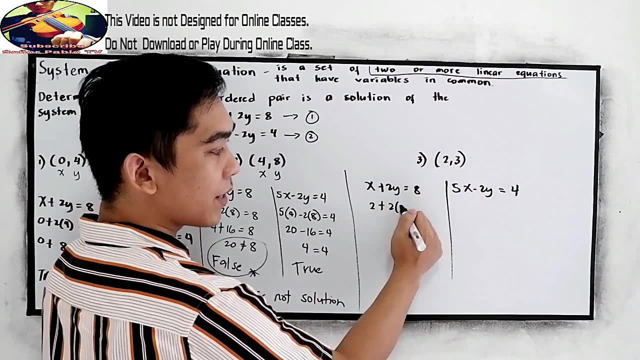 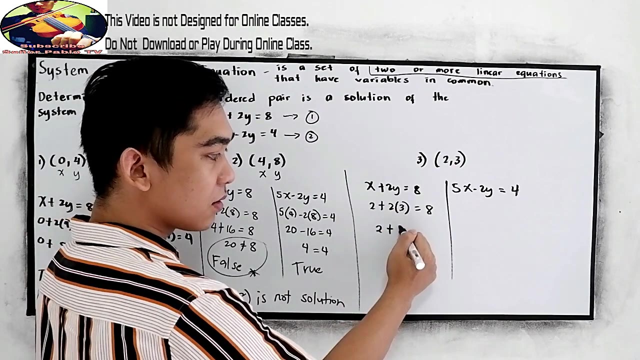 Copy: x plus 2y is equal to 8. And 5x minus 2y is equal to 4.. Now substitute So: 2 plus 2 times our y is 3 is equal to 8.. 2 plus 2 times 3, 2 is 6, is equal to 8.. 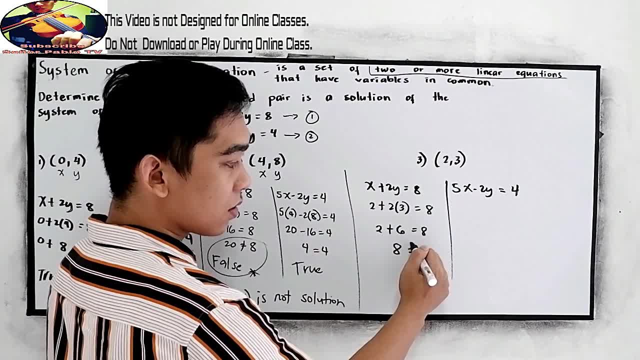 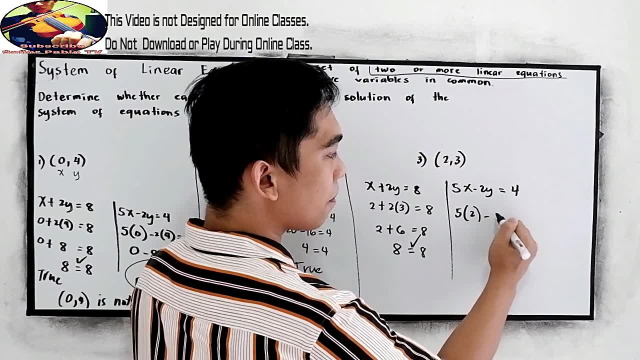 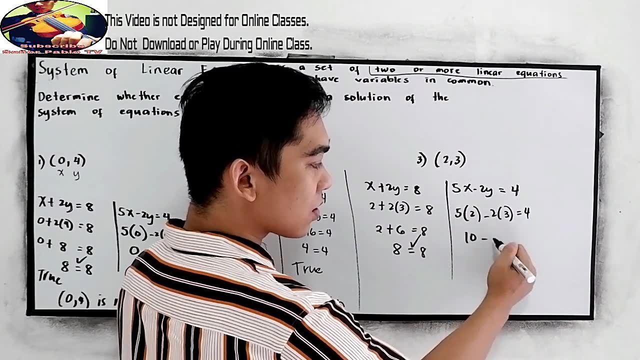 2 plus 6, 8 is equal to 8.. So it is correct. Now let us check the other equation: 5 times 2 minus 2 times 3 is equal to 4.. 5 times 2,, this is 10 minus negative, 2 times 3, times 3.. 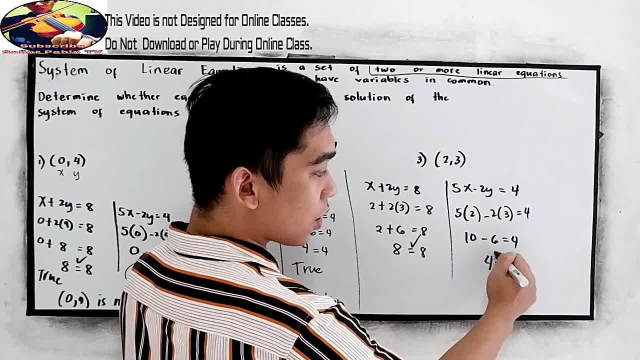 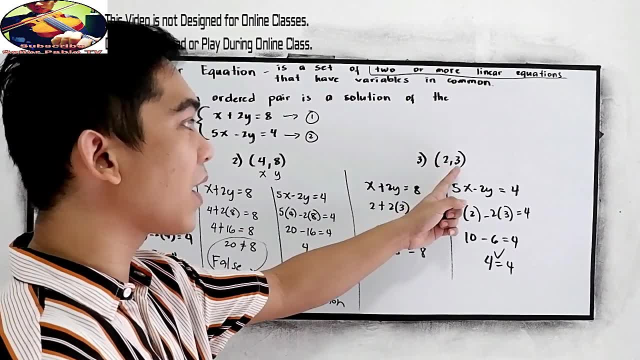 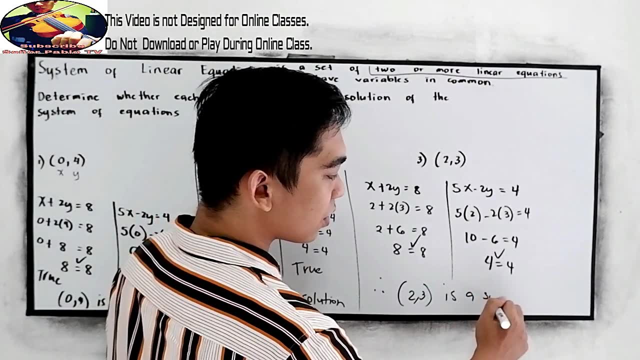 6 is equal to 4.. 4 is equal to 4, which is also true. So both equations are true when x is equal to 2 and y is equal to 3.. Therefore, 2 and 2 comma 3 is the solution. 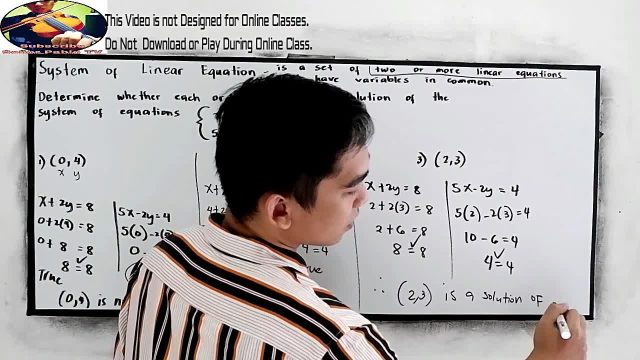 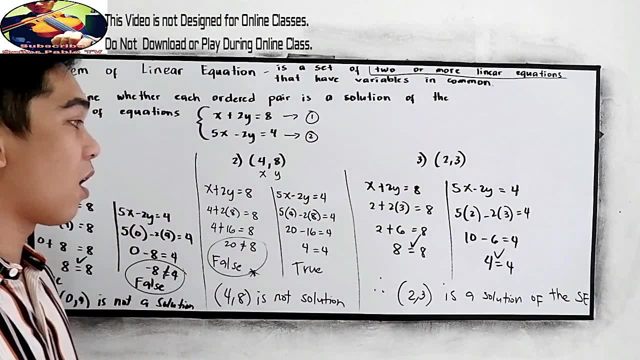 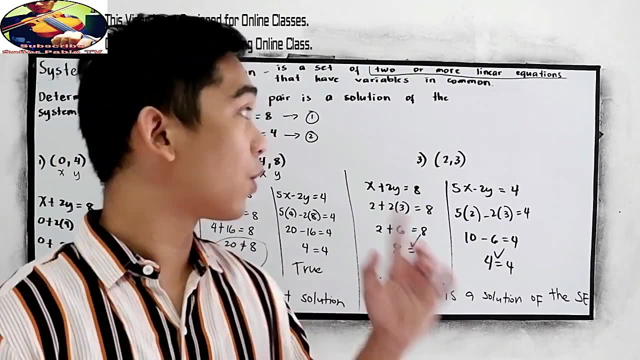 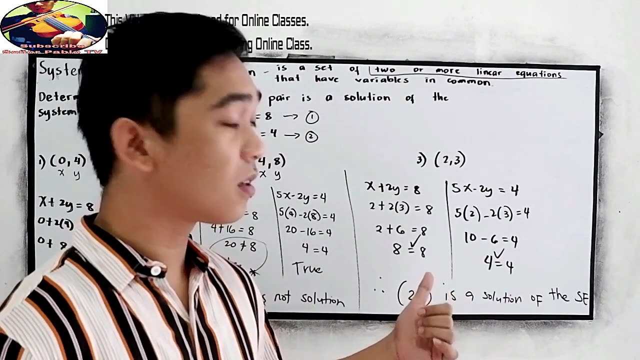 So we have the solution of the system of equations, The given system of equations. So you will be needing this process to check your answer in solving our linear equation with 2 or 3 variables. So you need to master the process in substitution. 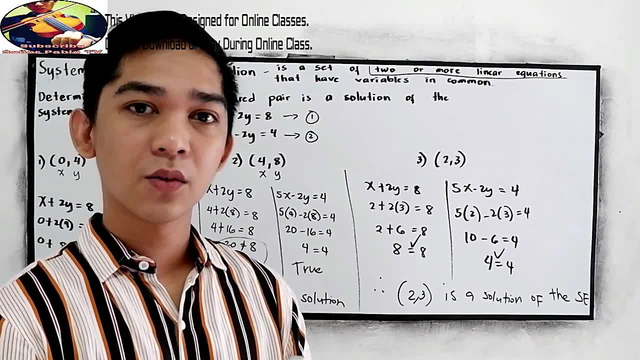 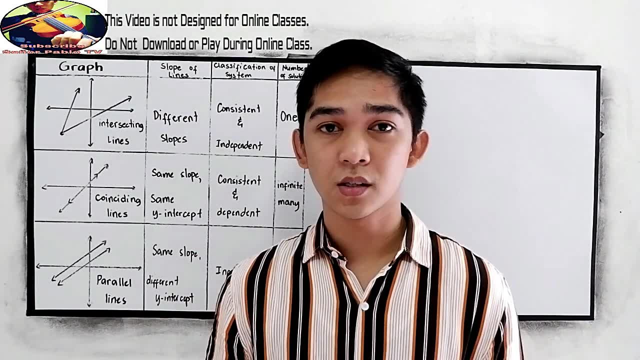 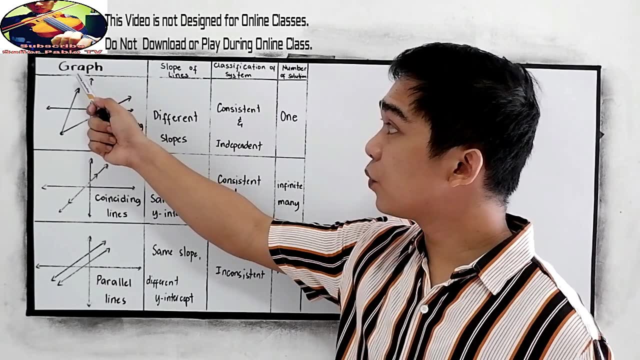 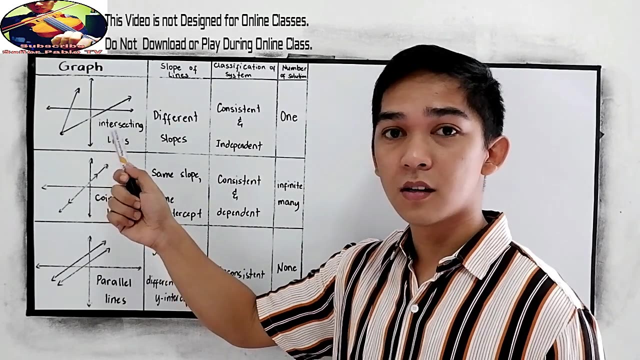 Now we are going to proceed in the graph of our system of linear equations. In system of linear equations, if we are going to graph, these are the things that you must know. So, if you will encounter a graph like this one, the intersecting line, that means the line, intersects at exactly one point. 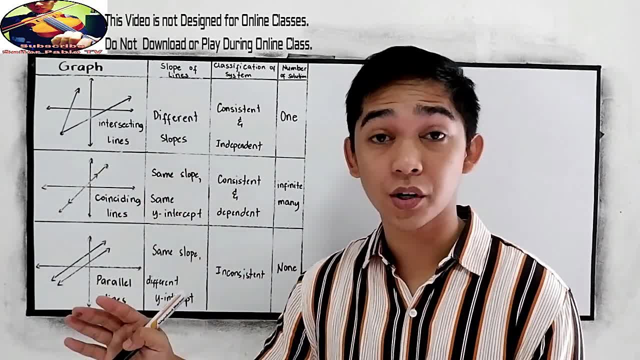 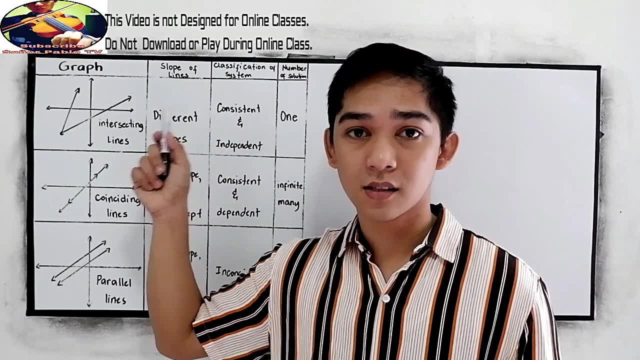 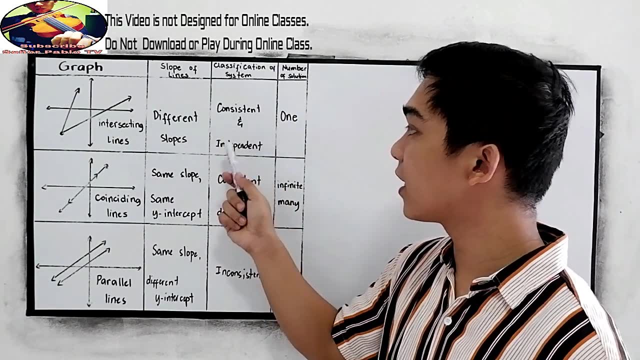 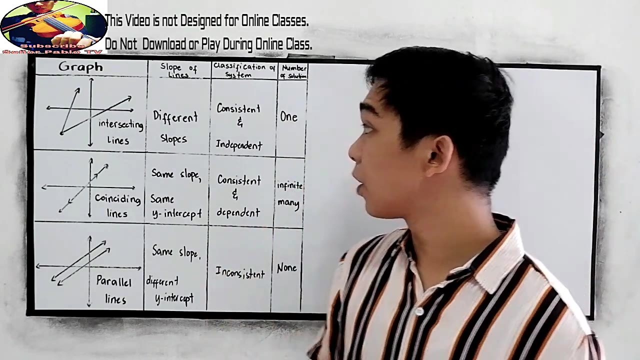 The slope of the lines are different, of course, Because the slope of this line is different from the slope of the second line And for the classification of system it is consistent and independent. And number of solutions we have only one, Or this is also called the unique solution. 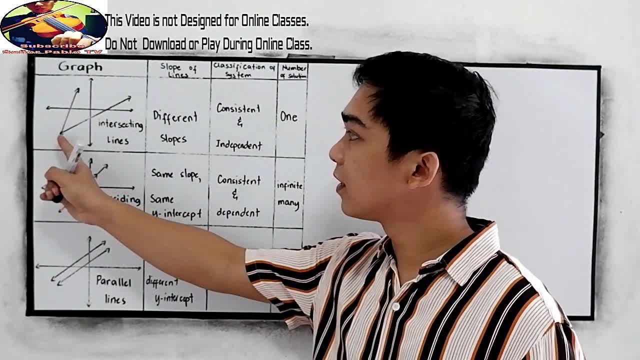 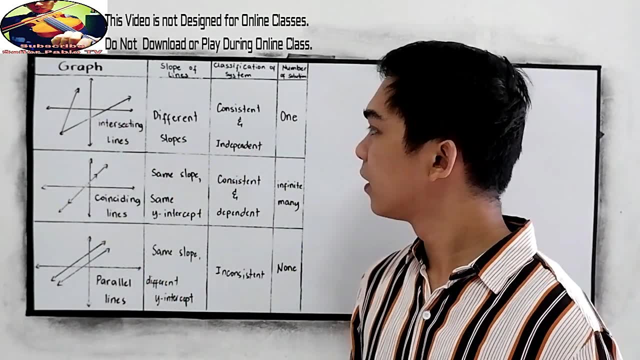 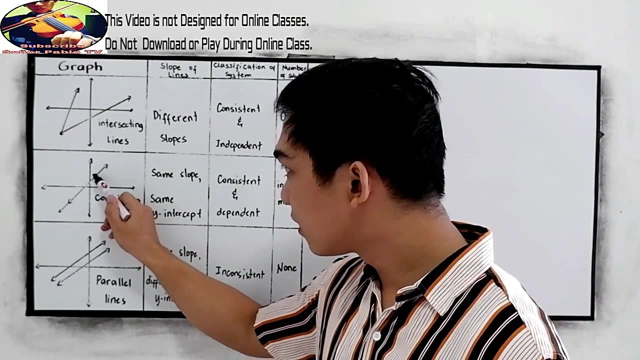 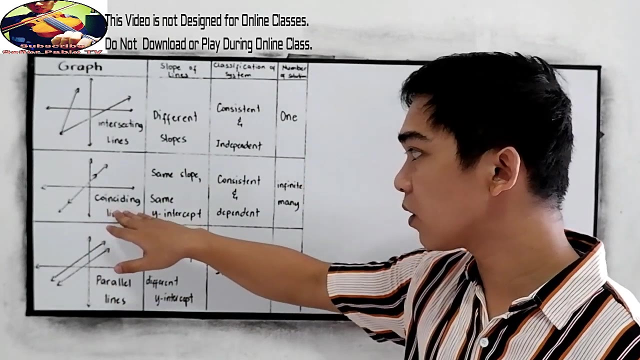 Because we only have a point, Exactly one point: that the two lines intersect, And that is our solution. And if you are going to encounter a graph like this one, So notice that the two lines coincide each other. That's why we call the coinciding lines. 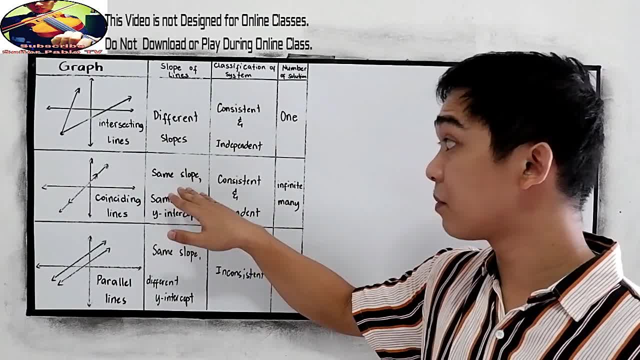 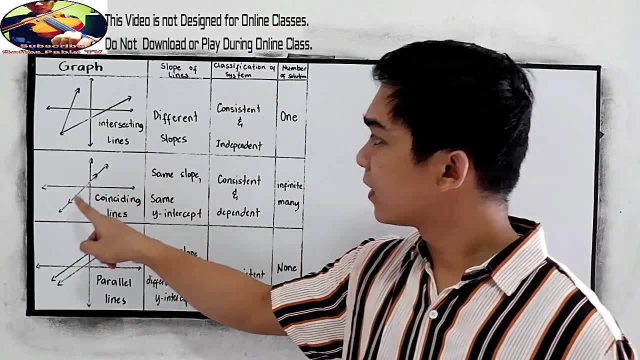 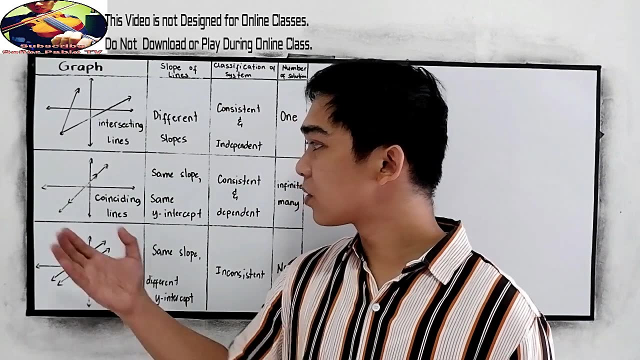 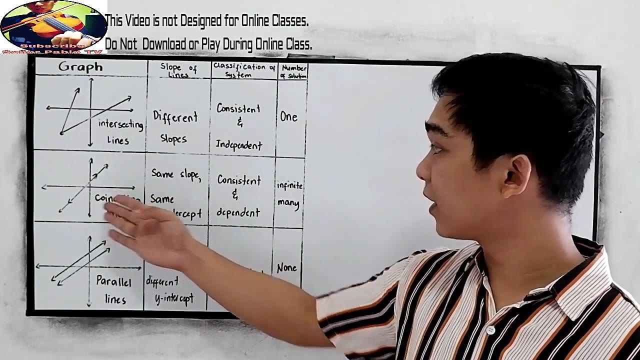 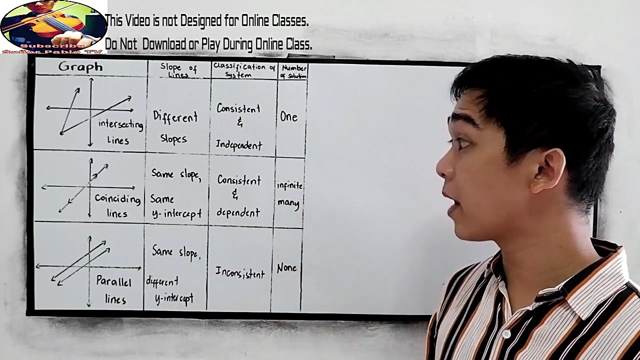 Our slope, same slope, And this MY intercept, Because, if you notice, This line is only one line that coincide, Because these are lines that coincide to each other And, of course, notice our line that is consistent and dependent And for the number of solutions, we have infinite, many solutions. 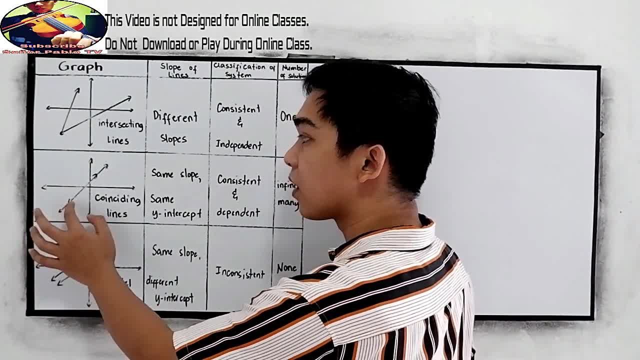 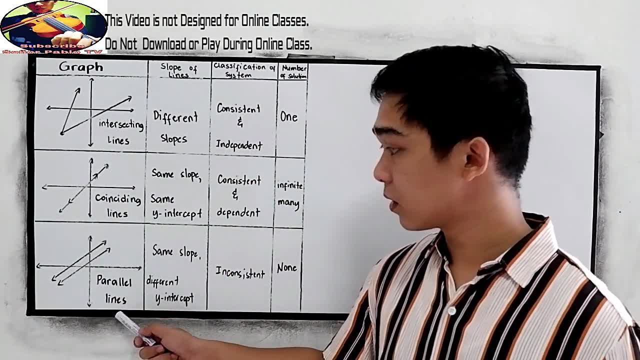 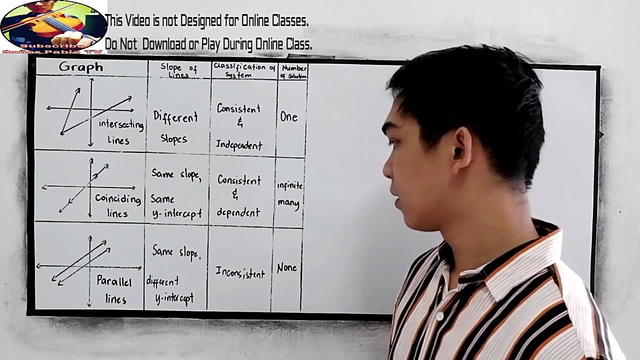 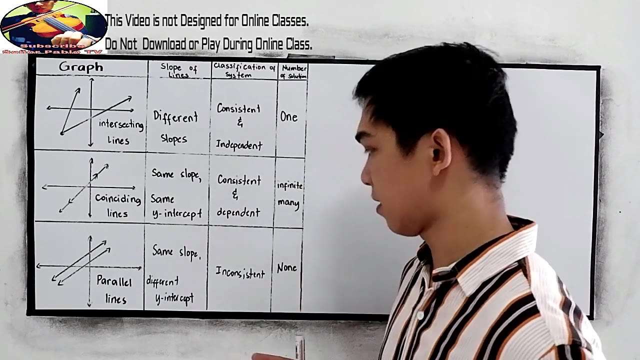 So if we are going to extend this, So we will come up with many or infinite many solutions. And the parallel lines, The slope are the same, but the Y intercept are different. And for the classification of system we have the inconsistent And the number of solutions. there is none. 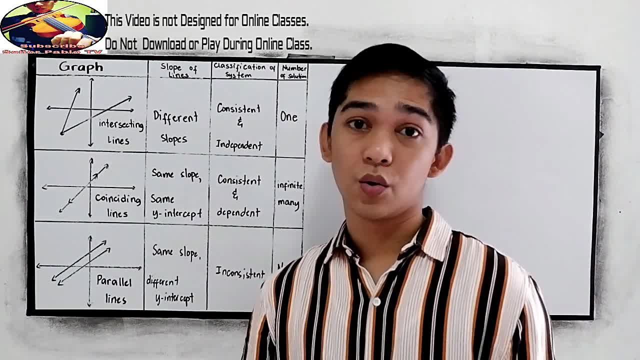 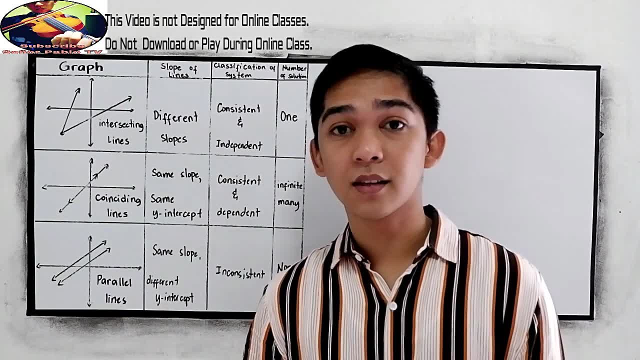 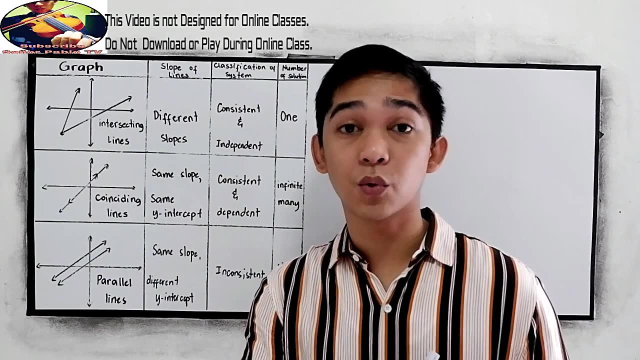 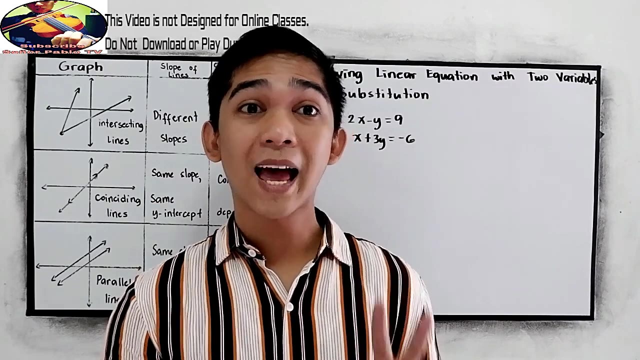 Because the two points will never touch each other. That's the parallel lines. To better understand, Kindly watch the next video, The solving linear equation with two variables, and it's graph: Solving linear equations with two variables. This time we will be focusing in substitution method. 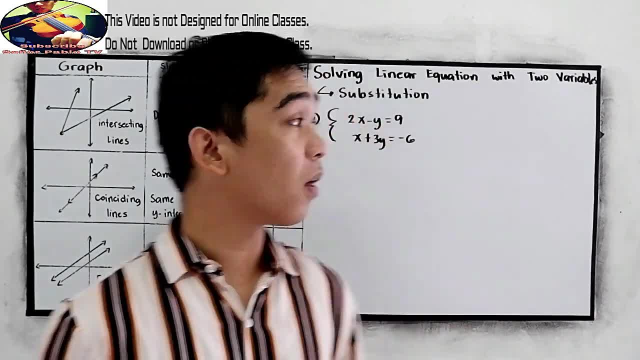 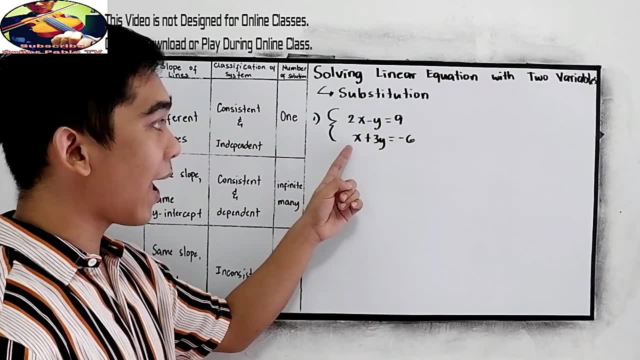 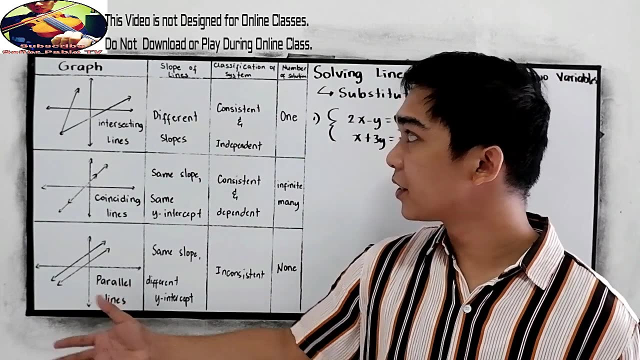 So let's have our example number one. The given equations are Two: X minus Y is equal to nine And X plus three, Y is equal to negative six. And notice in our board We have here the graph, This of the line classification in the number of solution. 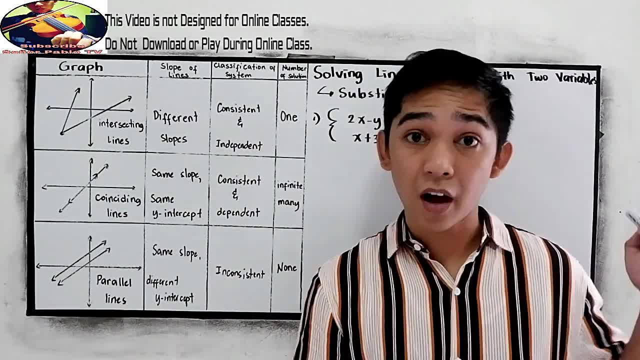 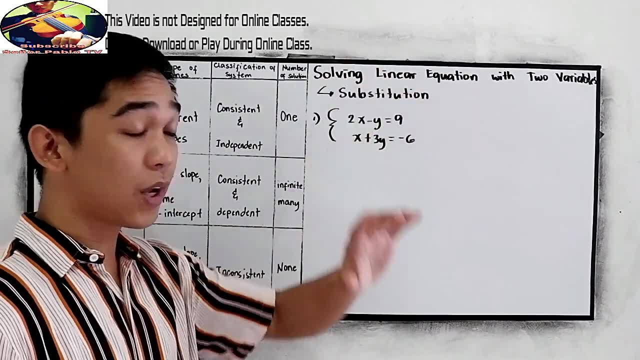 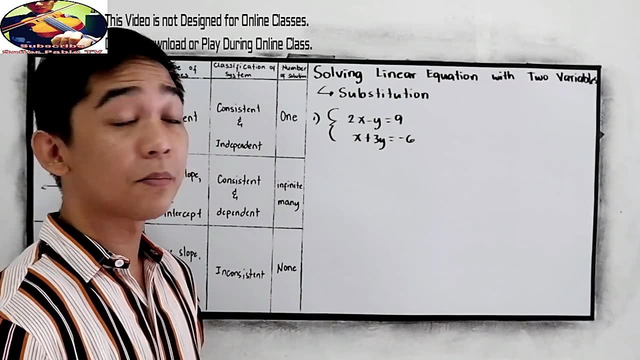 We will be needing this table In our graph later, So, aside from solving The X and Y using substitution, We can also graph this problem. Now let's try this Example Solved by substitution method, So of course we need to substitute. 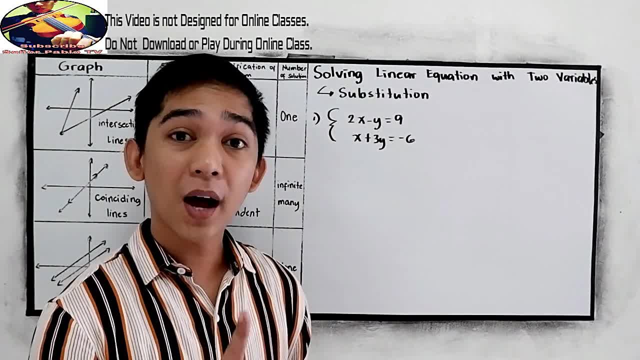 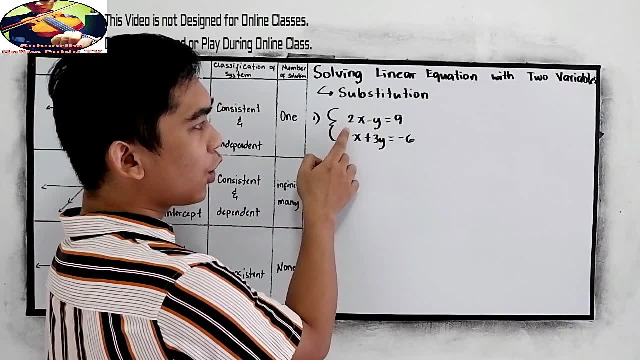 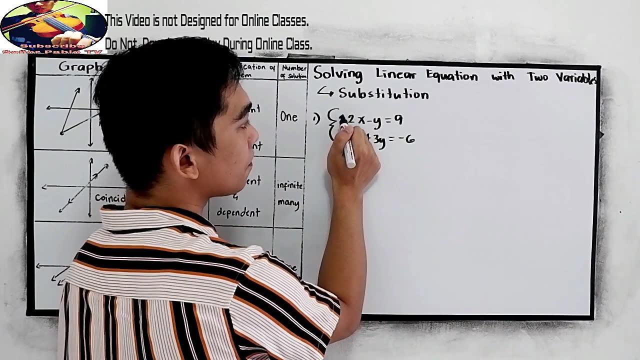 First, let us find the Value of X or Y. It's up to you. So, instead of the given, If we're going to Manipulate our equation one, Let's name it equation one, And this is equation two. Equation Y: 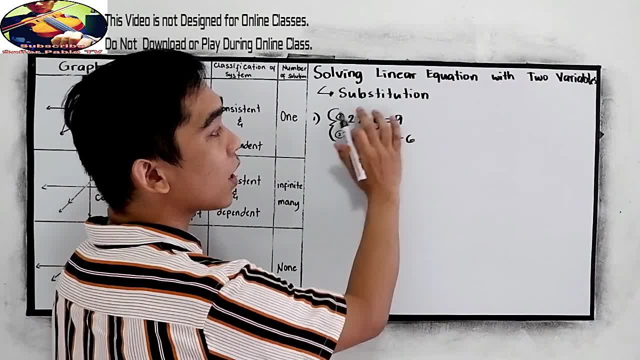 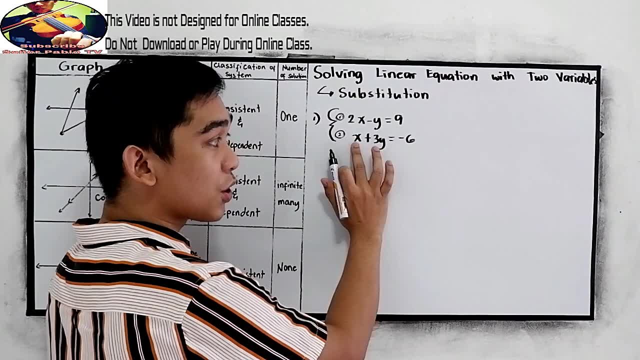 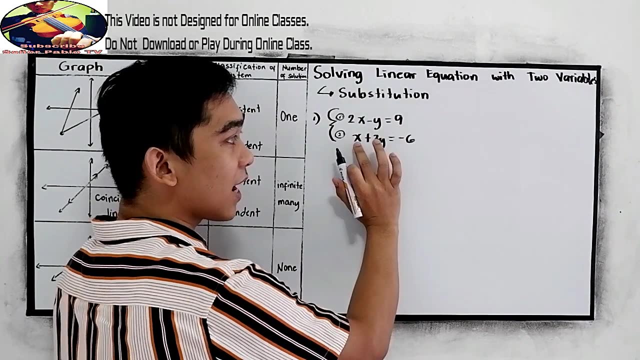 If we're going To use the addition property of equality, We can Find the value for Y. And in equation number two, Addition property of equality, We remove three Y on the right side We can get a value for X. Now let us find first the value of X. 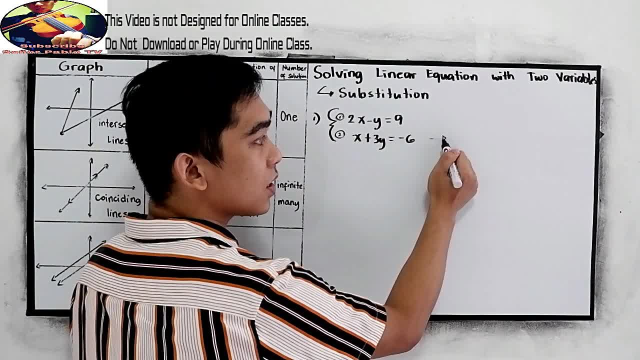 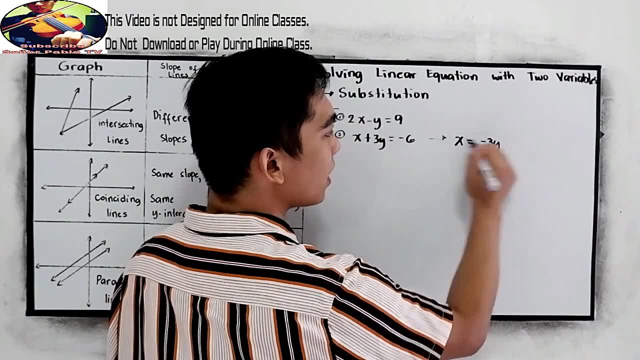 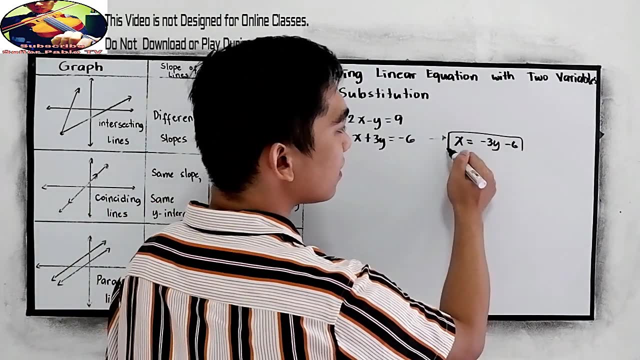 Let us use the equation number two. So this is also the same, as X Is equal to Negative three Y Minus six, We are the same. Now, after getting The value for X, We need to substitute in our: 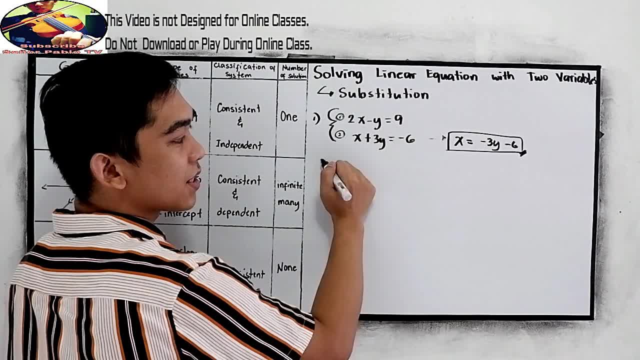 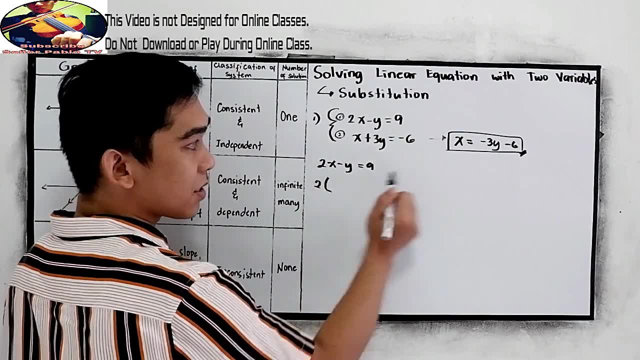 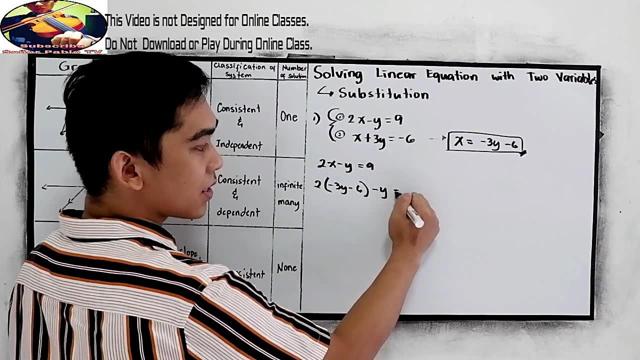 Equation number one. So the equation number one is: Two X minus Y is equal to nine. So we have a value for X. So two times Our X is Negative. three Y Minus six Minus Y Is equal to. 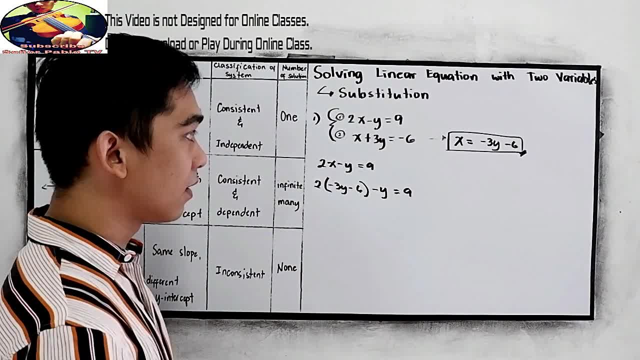 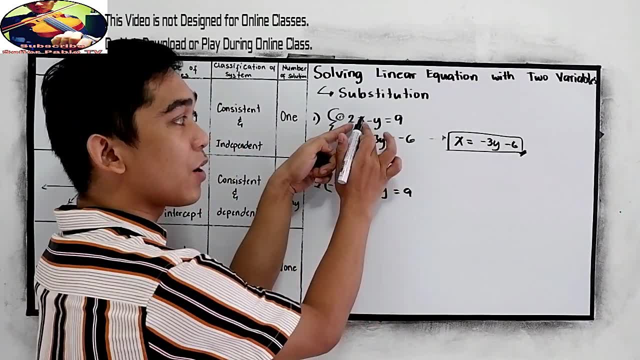 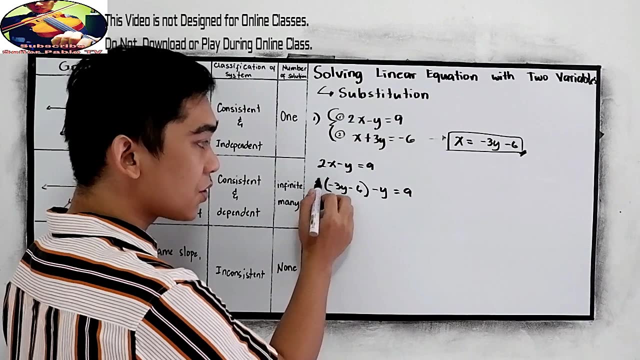 Nine Again, let us repeat. The value of X Is Three Y minus six. So the X in our equation one Just change into Negative three Y Minus six. Okay, Now Distribute Two times negative three Y. 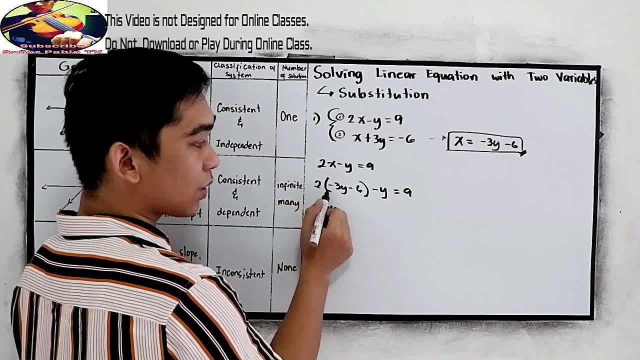 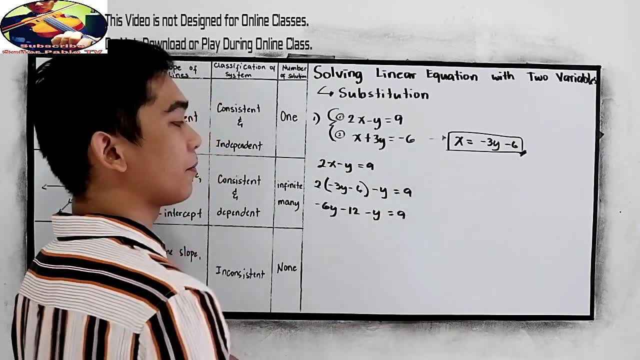 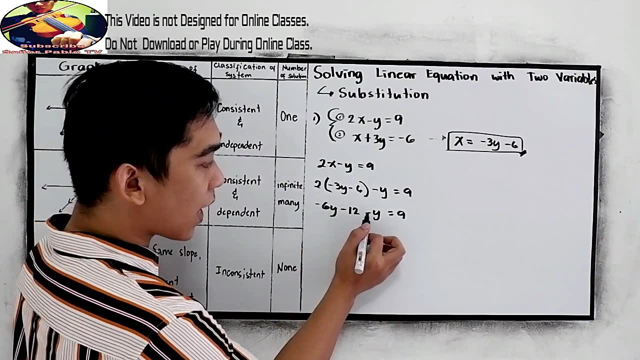 Negative six Y Two times Negative six. Negative twelve Minus Y Is equal to Nine. Now we are going to find the value for Y. So negative six Y Minus Y. Negative seven Y Is equal to. 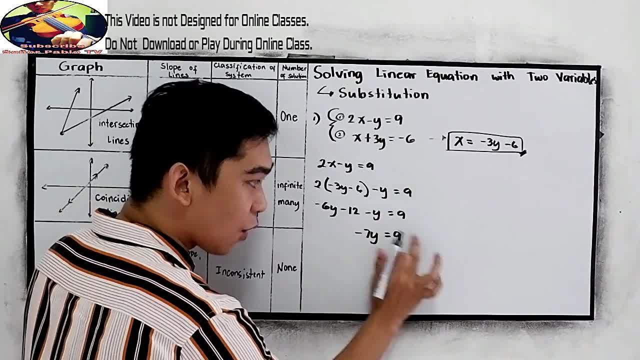 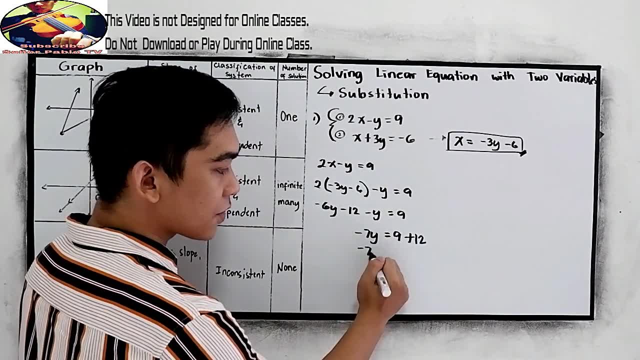 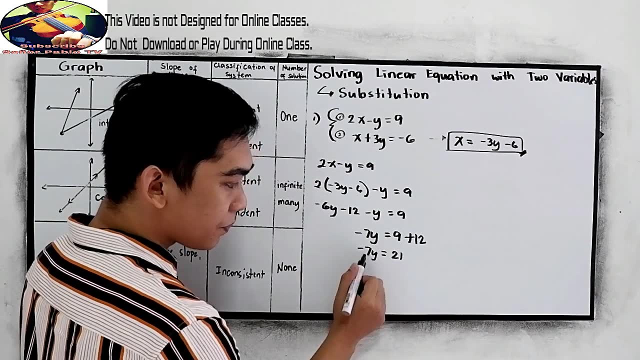 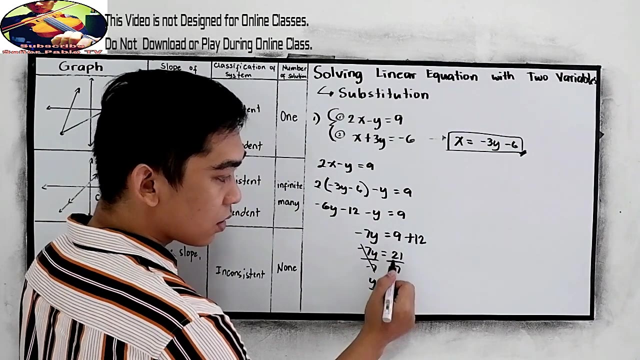 Nine, Addition: property of equality. I will move Negative twelve to the right, So that will become positive twelve, So negative seven. Y Is equal to Nine plus twelve. Twenty one Now we have Divide by negative seven, So Y is equal to. 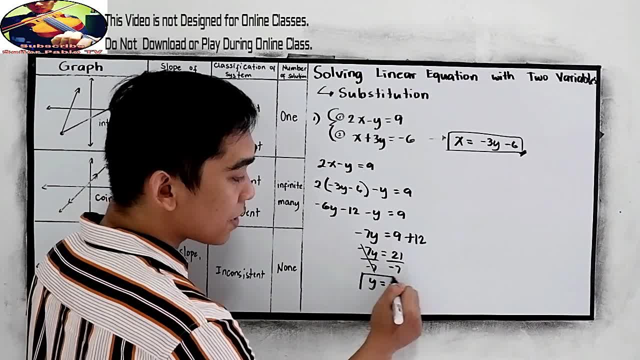 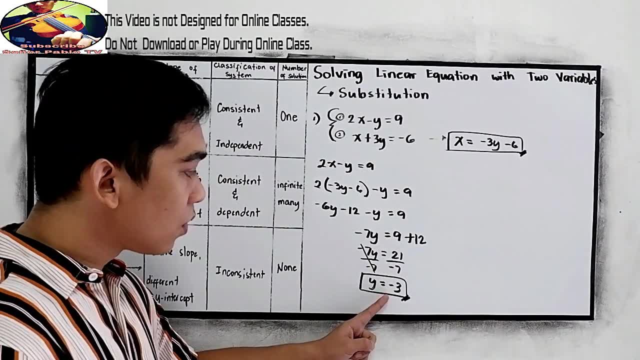 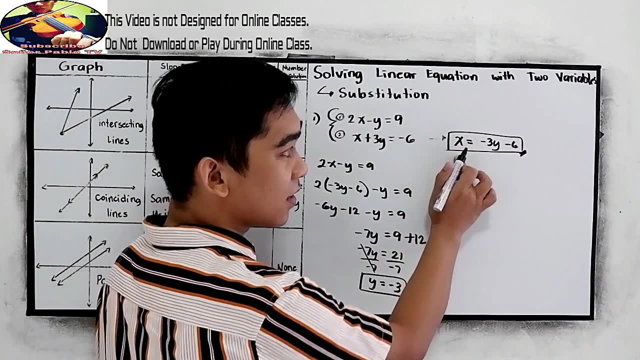 Twenty one divided by negative seven, Negative three. This will be The value For our Y. Now We have a value for Y. We can now get the value for X. Notice that X is equal to negative three, Y minus six. 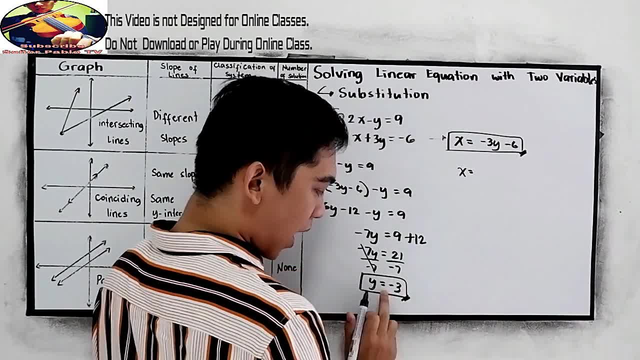 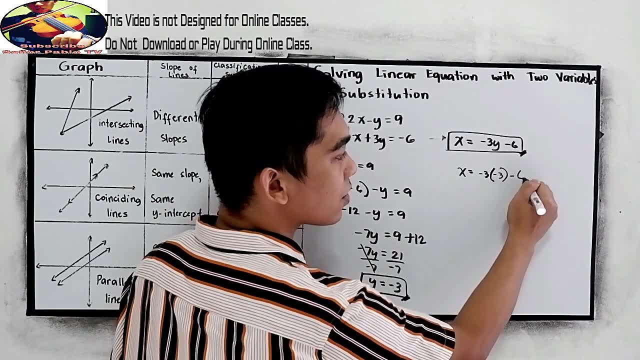 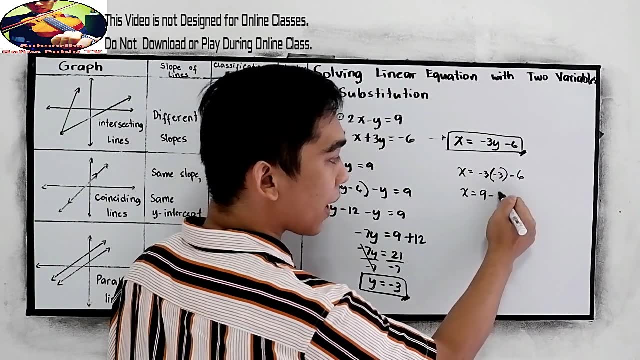 So all we need to do Is to substitute the value for Y. So X Is equal to negative three times Negative three minus six. So X is equal to Negative three times negative three. That is positive nine Minus six. 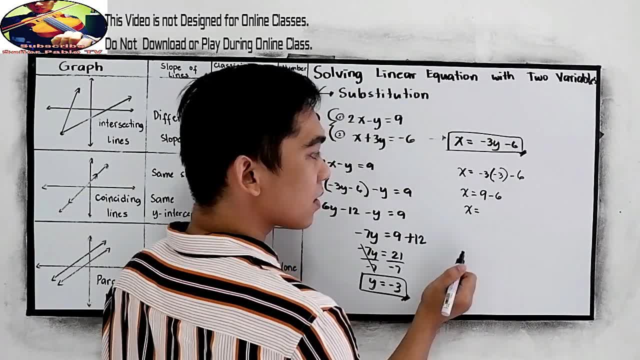 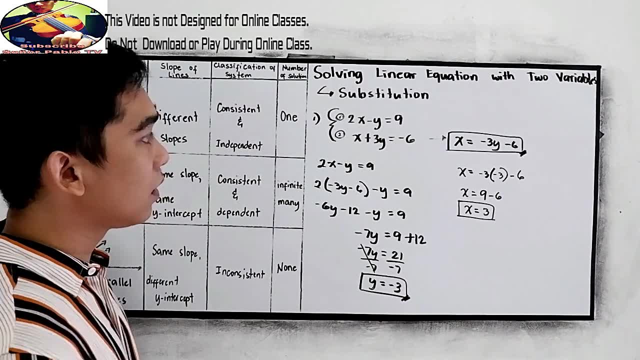 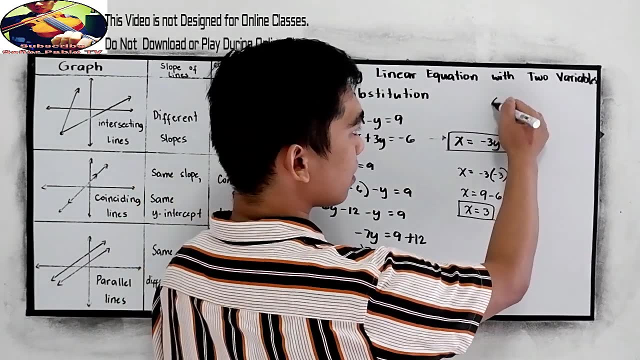 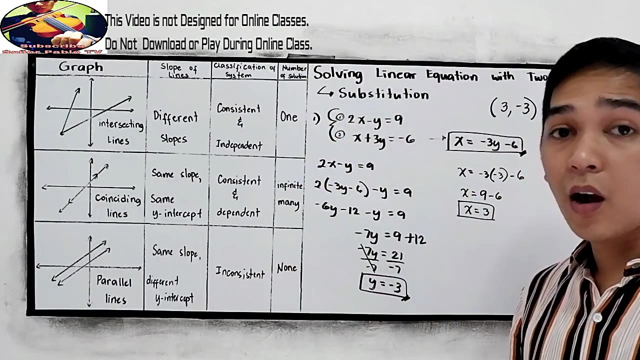 So X is equal to Nine minus six, That is three. So the solution of the System of equation Is: X is three, Y is Negative three. Now, If the question asks you to write The number of solution, 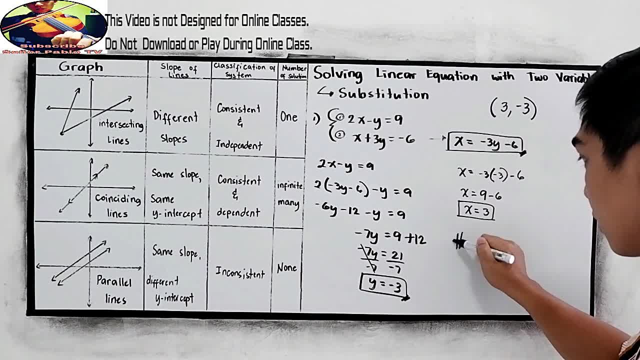 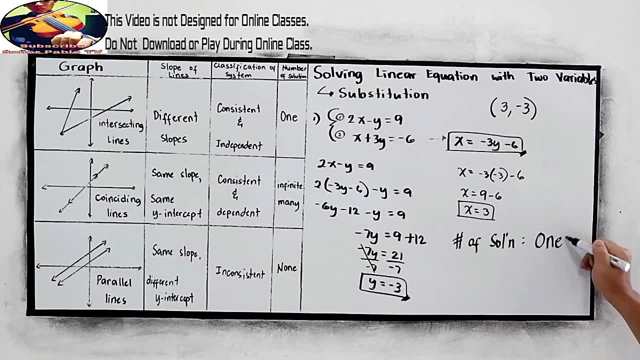 So number, Number of solution, You can write One- There is only one solution- And the classification of system. Classification Of system, We can write Consistent And Independent And, Of course, If you are going to try to graph this, 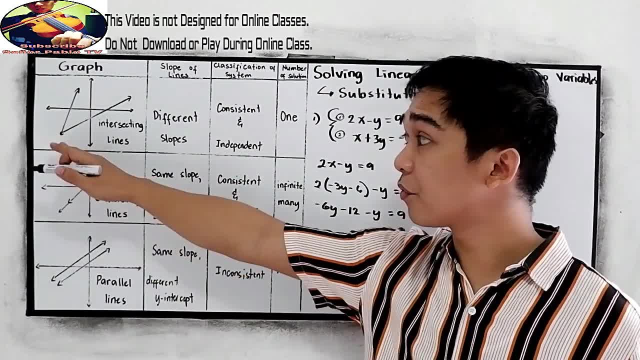 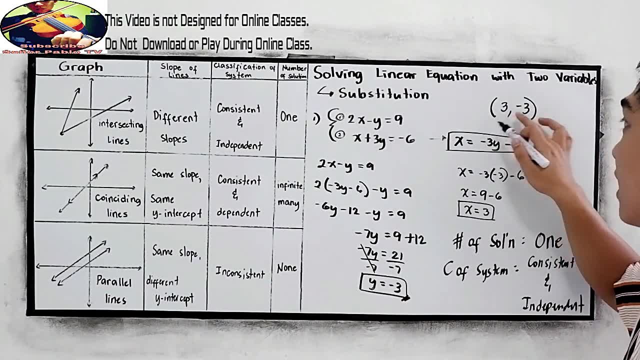 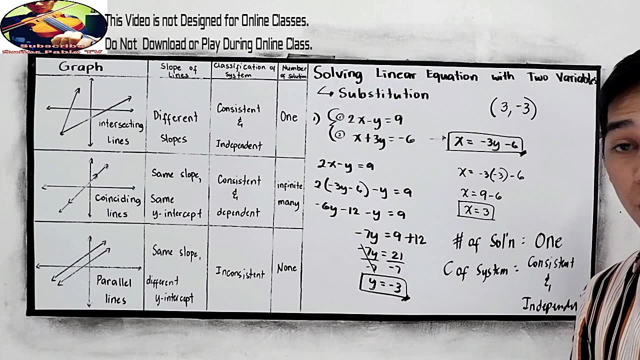 So This will be the outcome of your graph, Depending on the Solution of the linear equation. They will meet at three, Negative three. That will be the intersection Point of our Linear equation. So that's on how to solve. 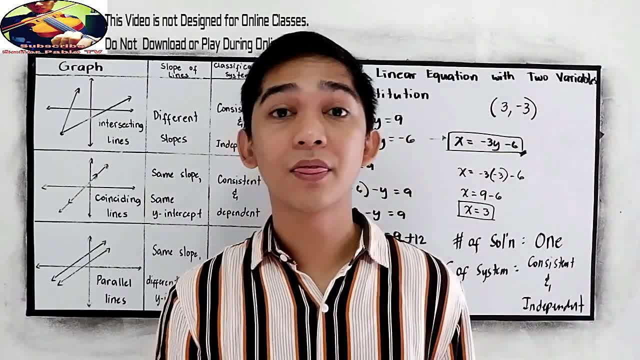 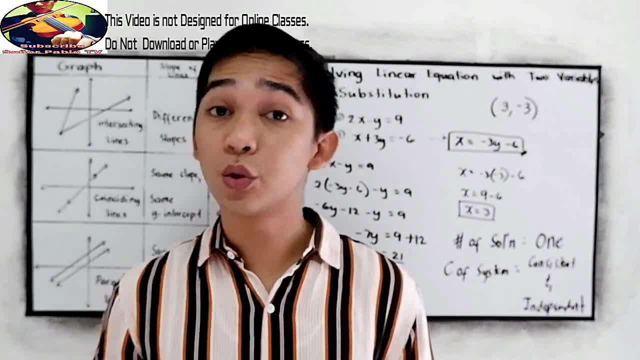 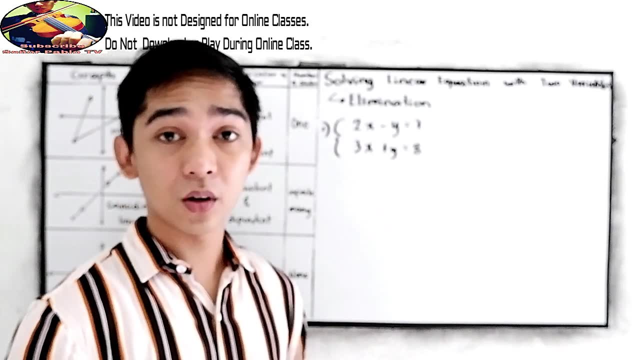 The linear equation Under the Substitution method. The next video will be Solving linear equation with two variables. We have the Elimination method Solving linear equation with two variables. This time we have The elimination method. So, after discussing the substitution method, 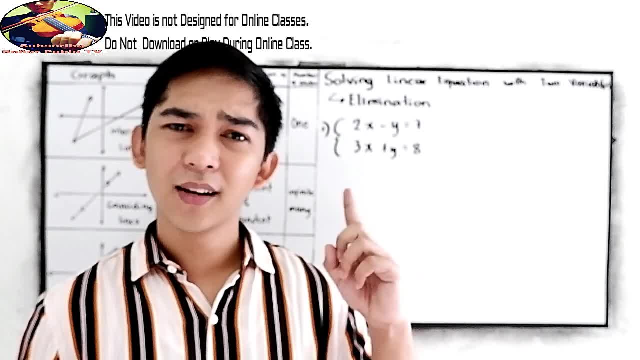 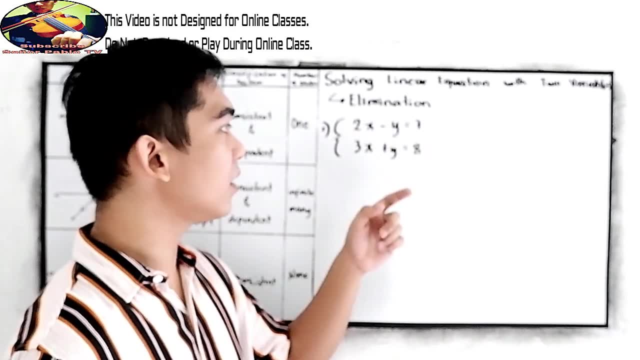 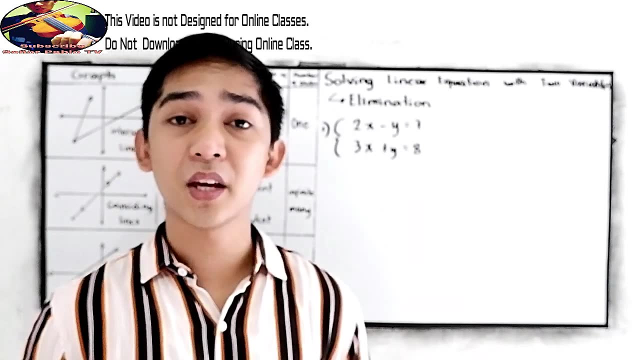 We have the elimination method. Let's have our first example. Our equation one is Two x minus y is equal to seven, And the second equation is Three x plus y is equal to eight. So, since we are in the elimination method, 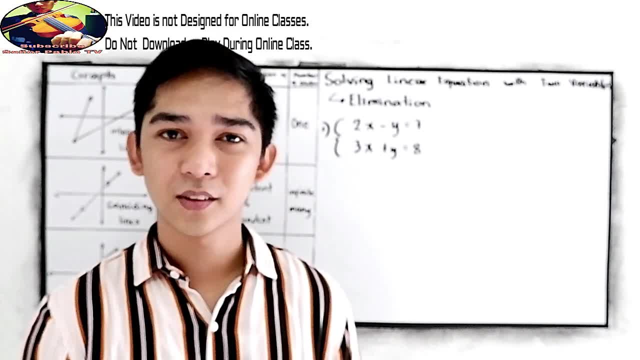 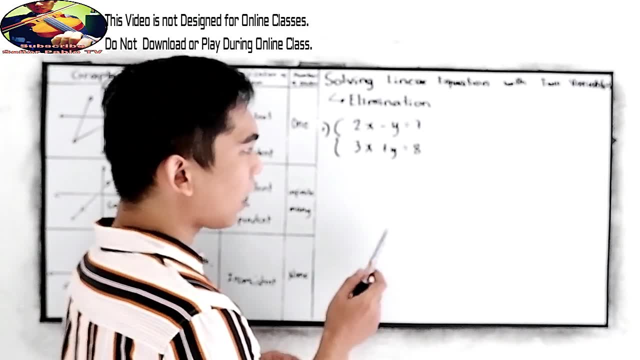 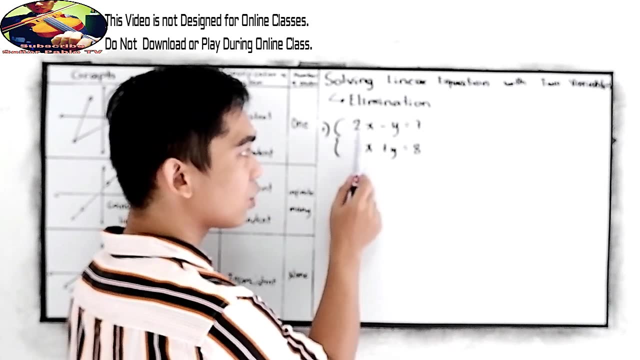 We need to eliminate one of our variables. Let's say we're going to eliminate our x, So our goal is: The coefficient must be the same. In this case they are different: Two x and Three y. So all we need to do 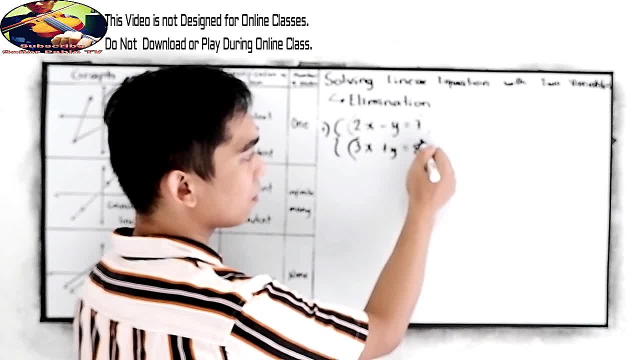 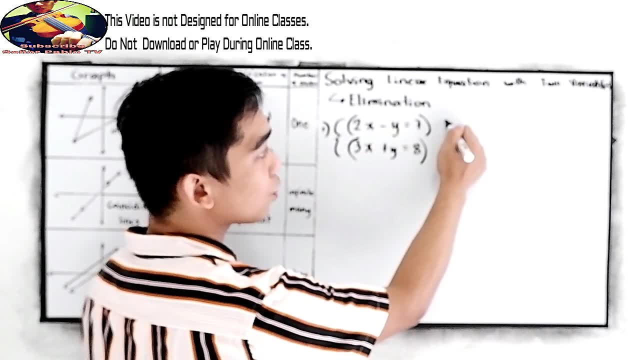 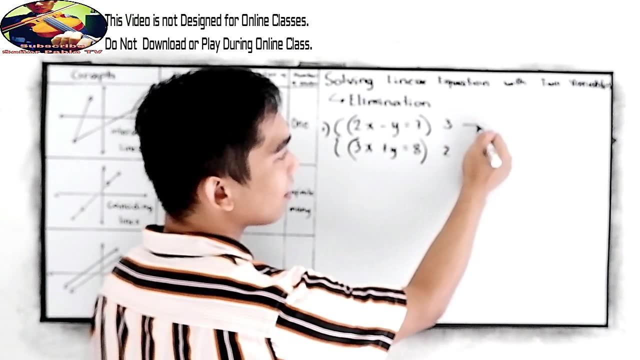 Is To make them The same. Okay, So We need to multiply In our equation one To three, And in our equation one, Multiply it to two, So that The equation will be Two x times three, That is six x. 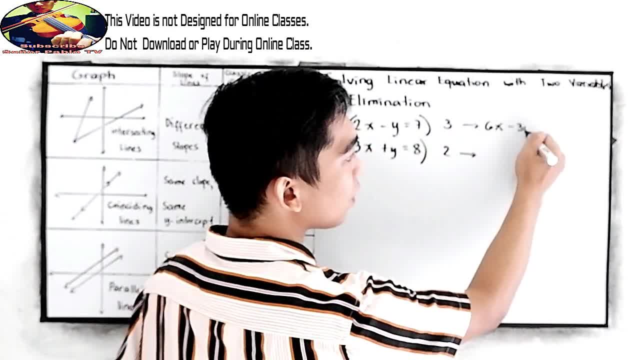 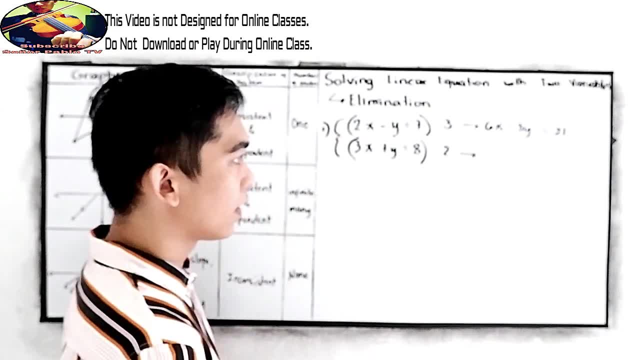 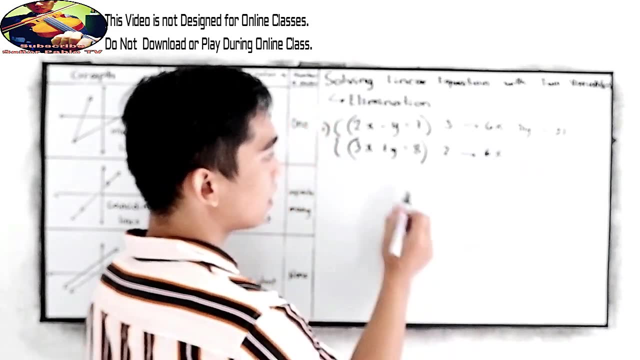 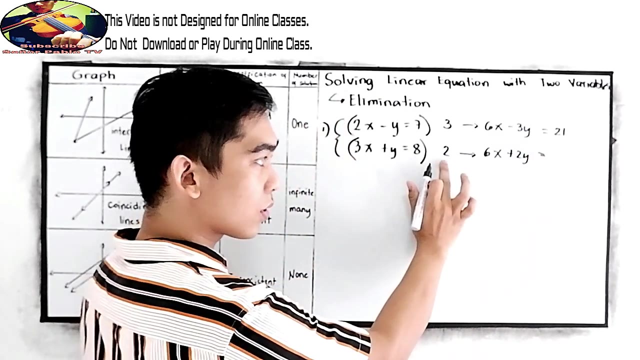 Negative y times three. Negative three y Is equal to Seven times three. Twenty one. Second equation: Two x times two, That is six x Y times two. That is positive two y Is equal to Two times eight. 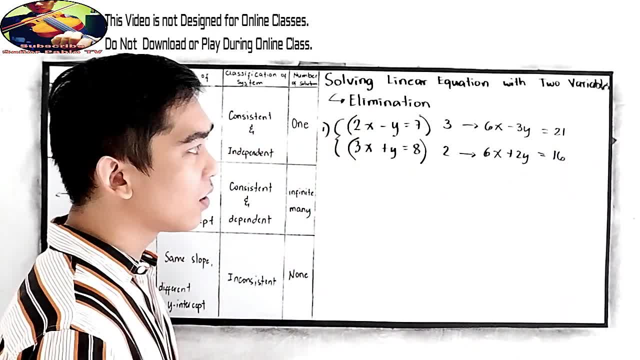 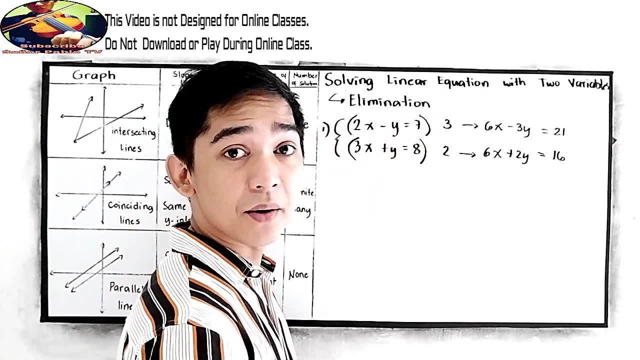 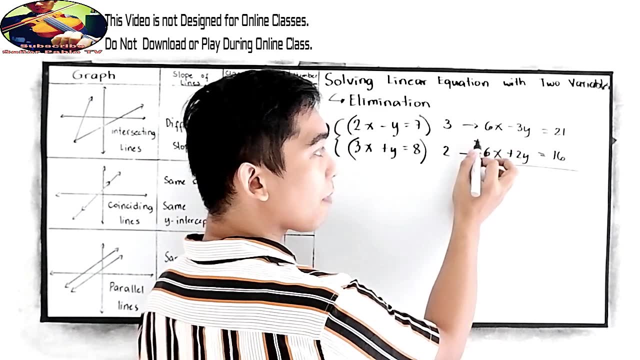 Sixteen, Notice that Our coefficients In our x Are the same, So To eliminate that We need to subtract: Okay, So six x minus six x, That will be Zero, Or we can just cancel that out. 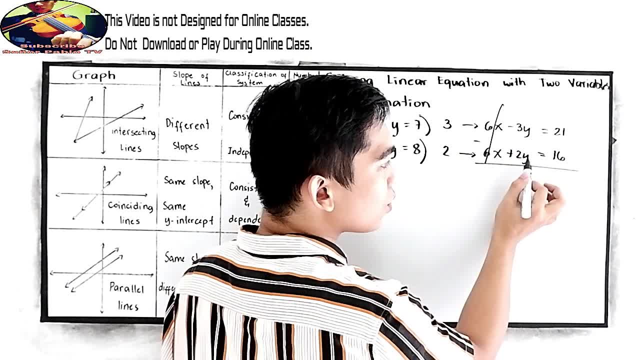 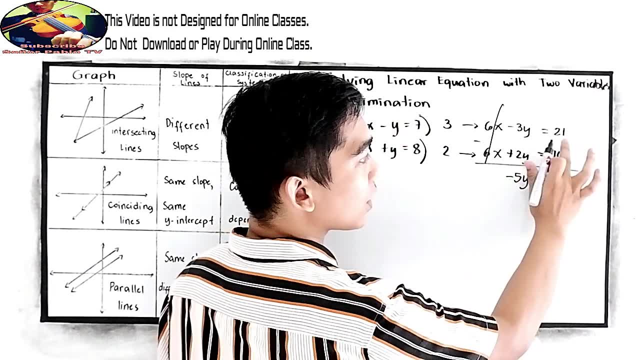 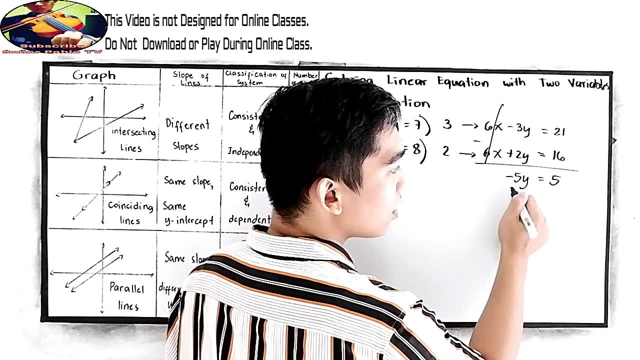 Now Negative three: y Minus two y, That is negative five. y Is equal to Twenty one minus sixteen, That is five. We need to get the value for y, So We need to divide by negative five. Negative five: 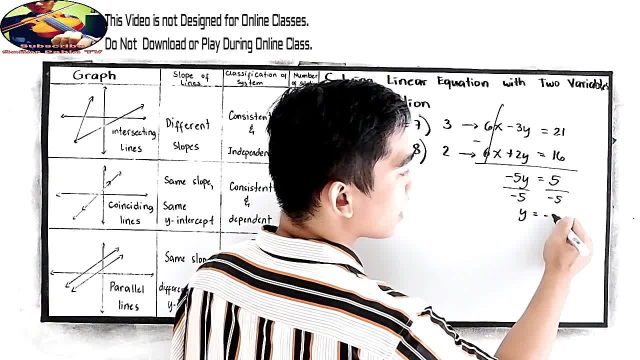 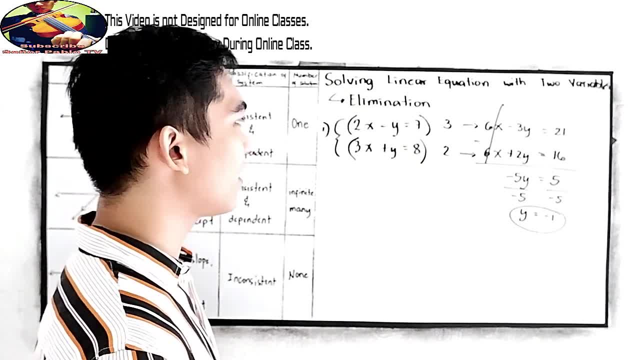 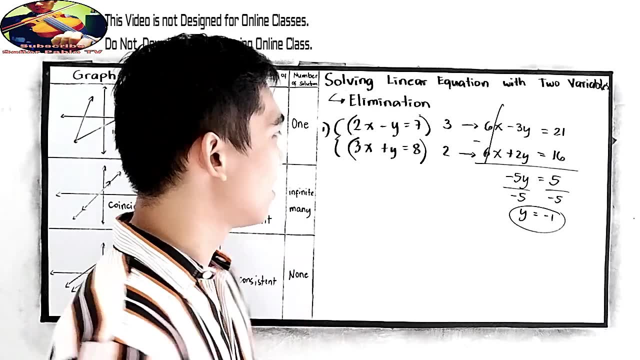 So y is equal to Negative one. Okay, Next We need to find The value for x. So we need to eliminate now The y. So we have Just copy: Two x Minus y Is equal to seven. 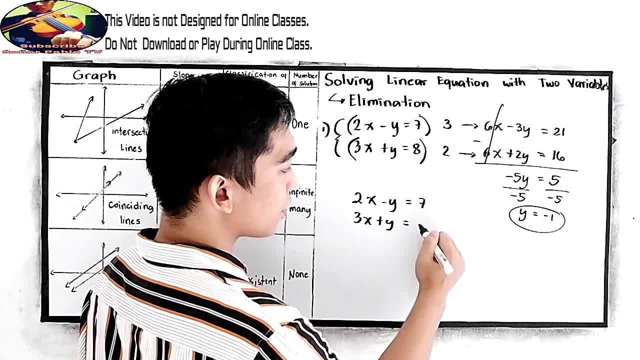 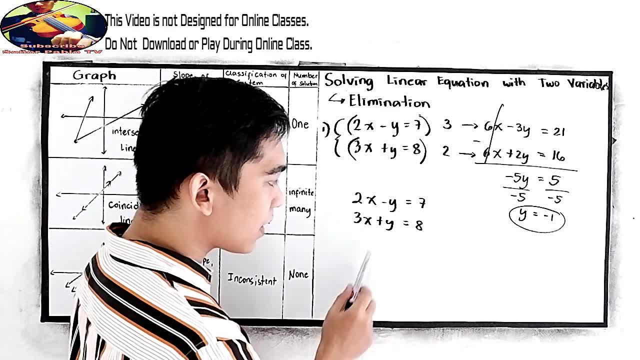 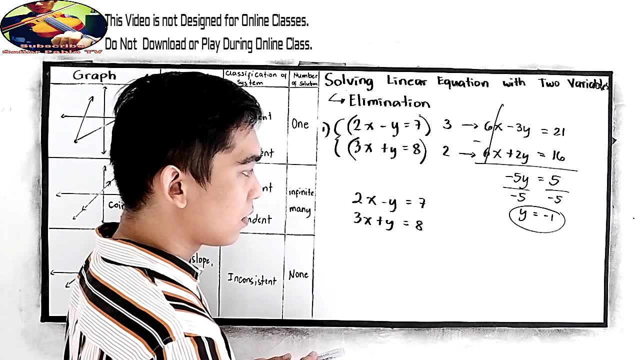 And Three x Plus y Is equal to Eight. Check the coefficient of y. We have negative one And Positive one, So they are the same. They are just different in their sign, But our coefficient here is one. 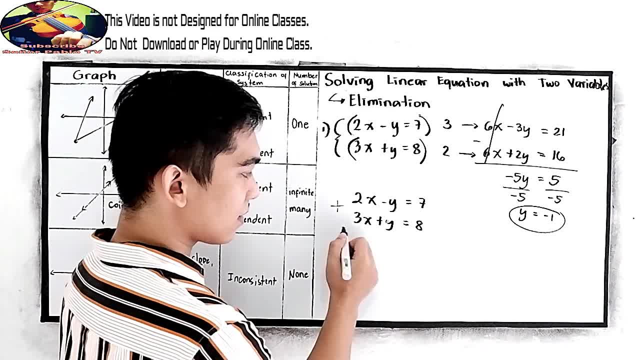 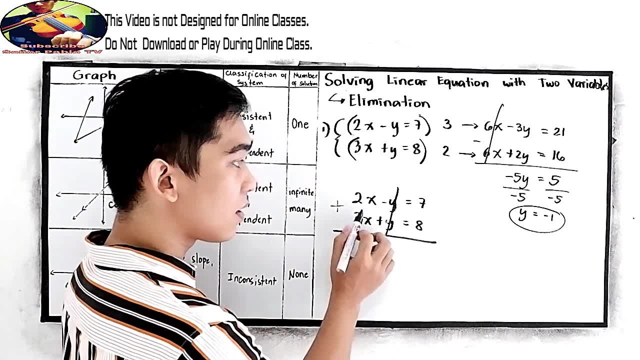 And one. So If we are going to add that Negative one Plus Positive one, That will give us zero. So it will be cancelled out. Now we have Two x Plus three y, That is, five x And seven plus eight. 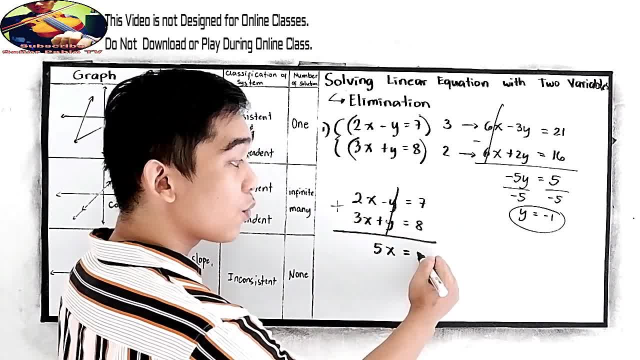 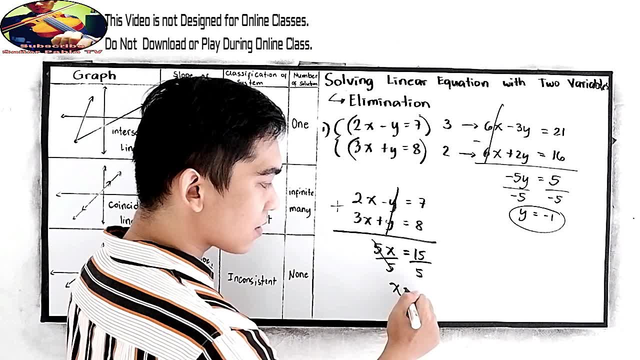 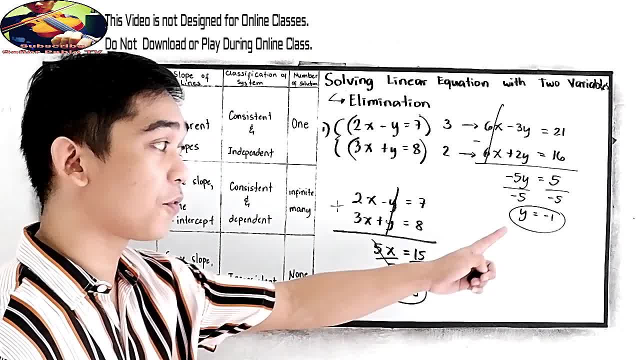 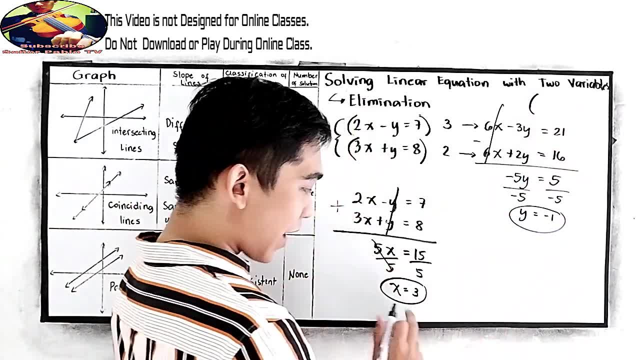 That is Okay. Now we have the values for x And for y. So our Solution now Is: Our x Is three And our y Is Negative one. Okay, Now let us try To substitute in our 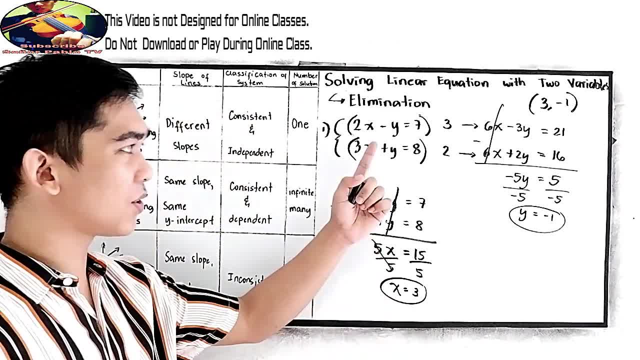 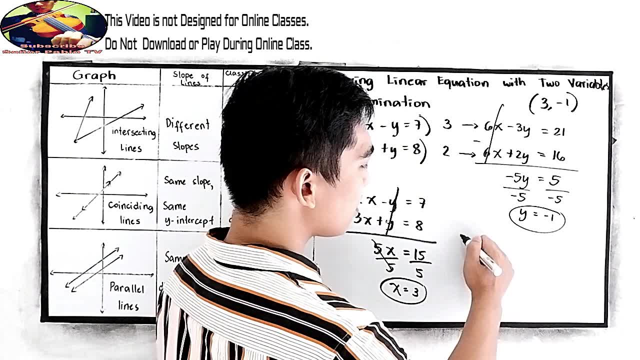 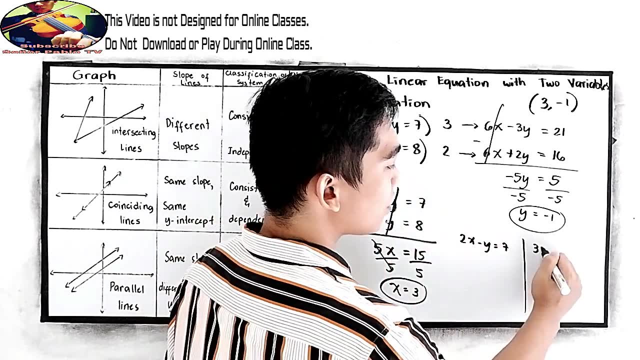 Equations To check your answers. So Equation one And Positive one That is Negative, one That is Negative one, Negative one That is Positive one. So Two times Three, So Two x. 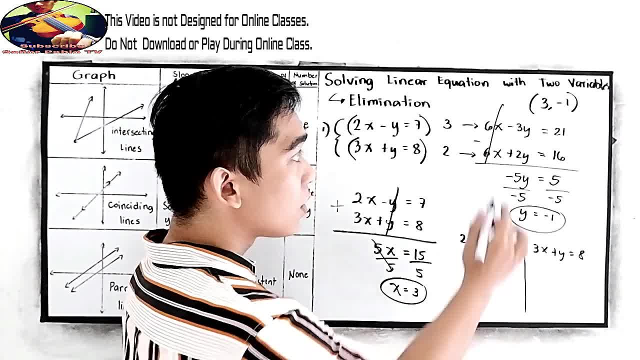 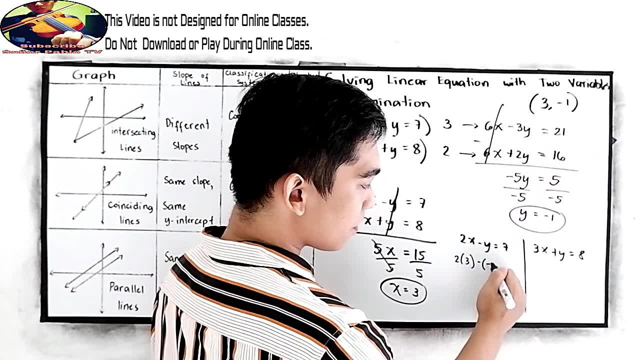 Minus y Is equal to Seven And the equation two, Three x Plus y Is equal to Eight, So X is three. So Two times Three Minus Y is Negative, one Is equal to. 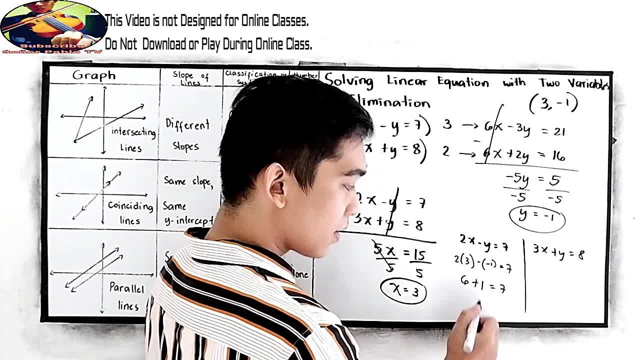 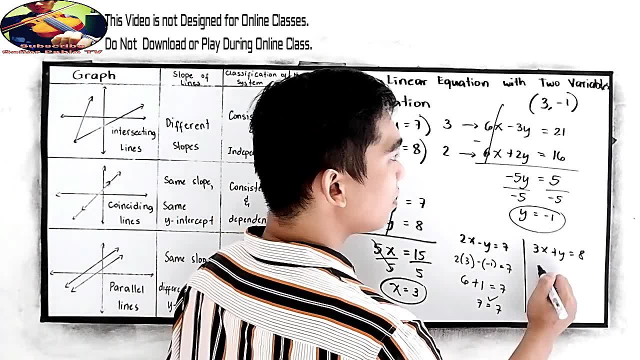 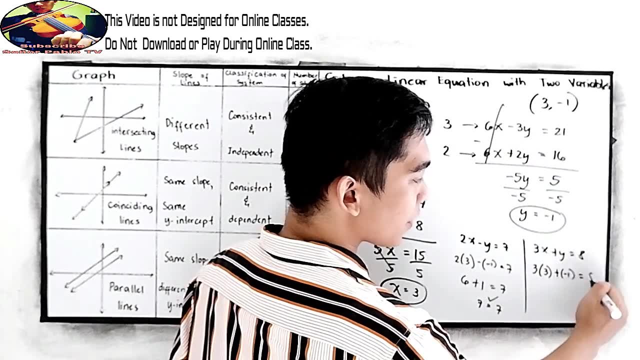 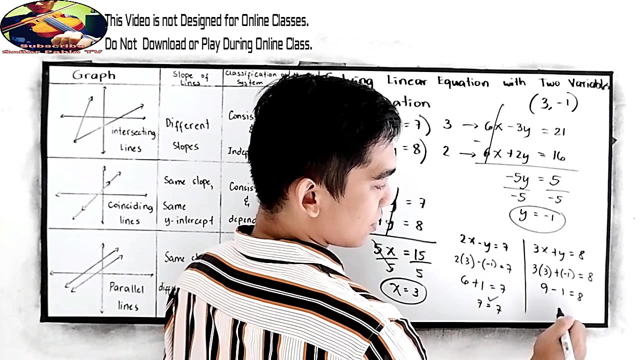 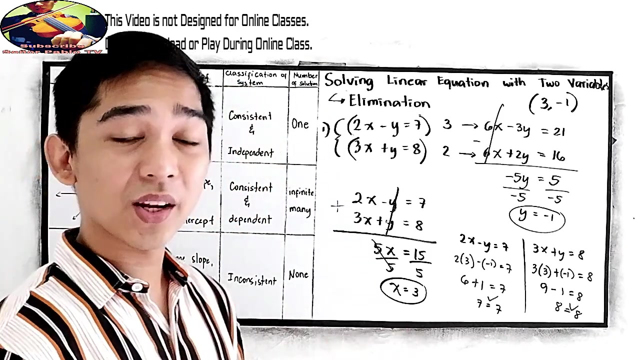 Seven Two times Three, That is Six, equal to 7.. True Now, 3 times 3 plus negative 1 is equal to 8.. 3 times 3,, that is 9, minus 1, is equal to 8.. So 8 is equal to 8.. Okay, correct, True. Now, if the patient asks you: 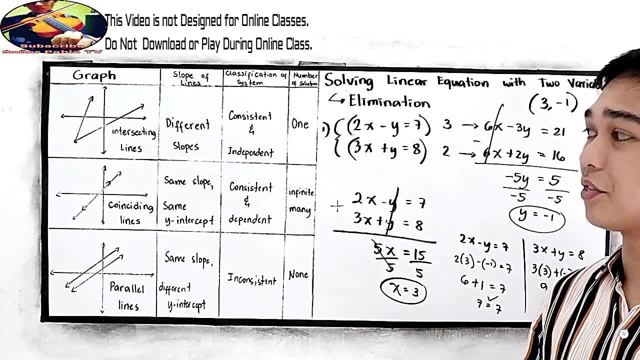 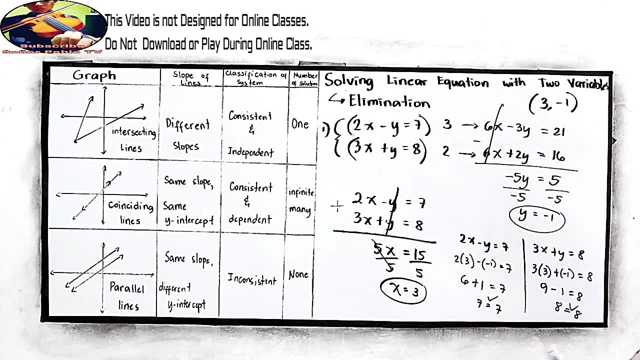 to determine the graph: is it intersecting, coinciding or parallel? So, since we have one solution, so it is intersecting- Intersecting And the classification of systems. we have the consistent and independent And the number of solutions. you have one or the unique solution. 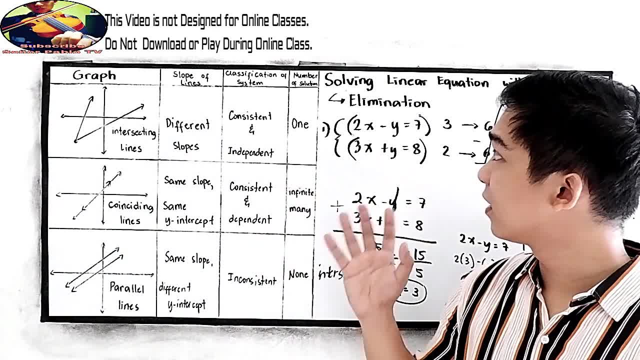 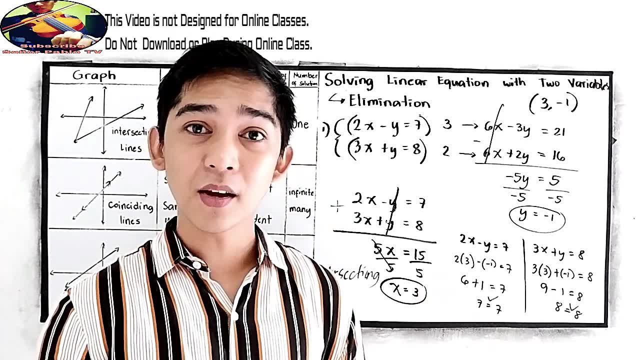 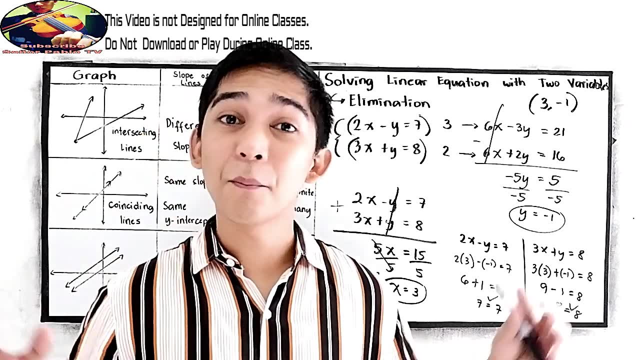 That is the use of our table. The shortcut here in elimination method is that you're going to manipulate our equations so that our coefficient will be the same. then you will be. you need to cancel that out. For our next video, we will combine the elimination. 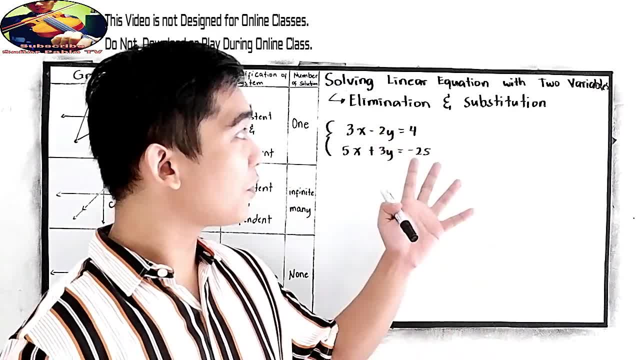 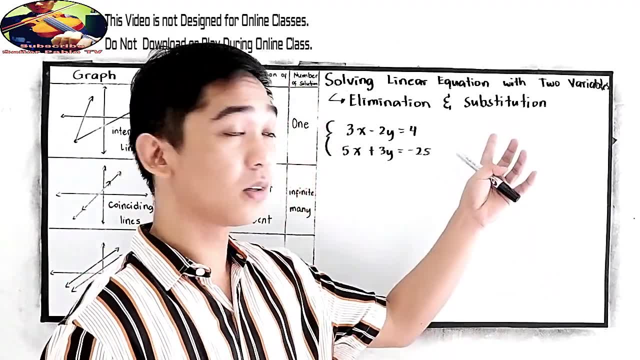 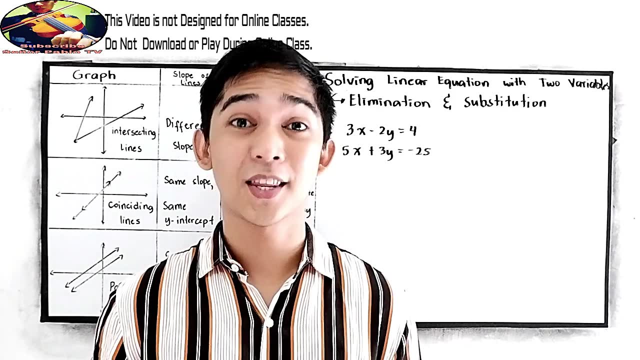 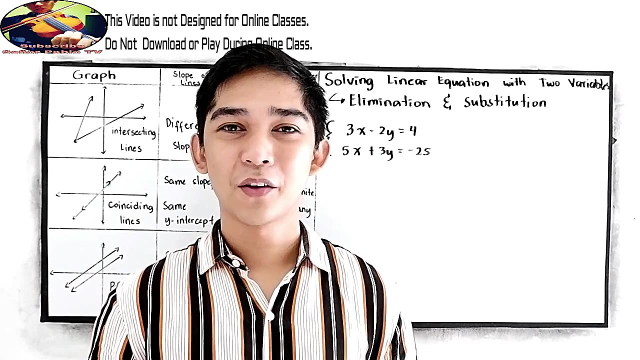 and the substitution method. Solving linear equation with two variables. we're going to use the elimination method and the substitution method. Okay, So make sure that you watch our videos in substitution method and elimination method. This time we're going to combine the two methods, So if you find this easy, then you. 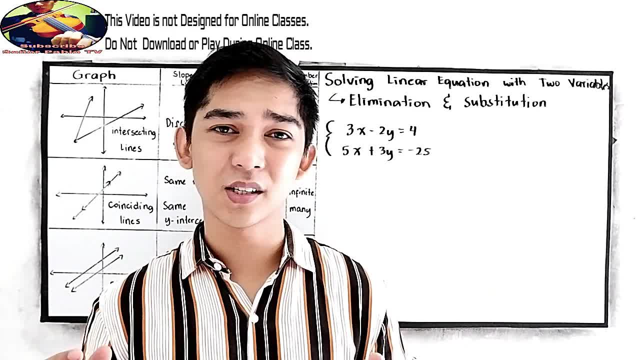 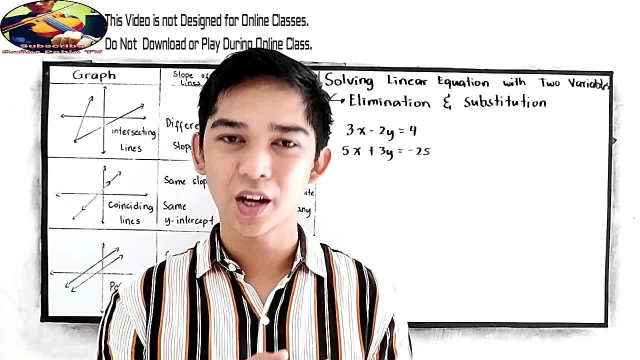 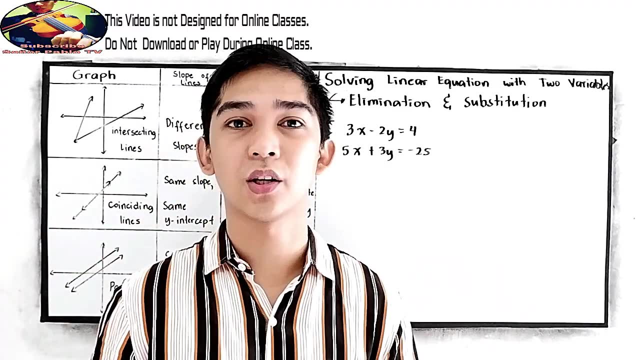 can use this process. But if you are confident to use the substitution method, then go ahead. And for elimination method. if you are confident to use that, you can use that. But a lot of people don't like the combination of elimination and substitution because they find it the easiest. 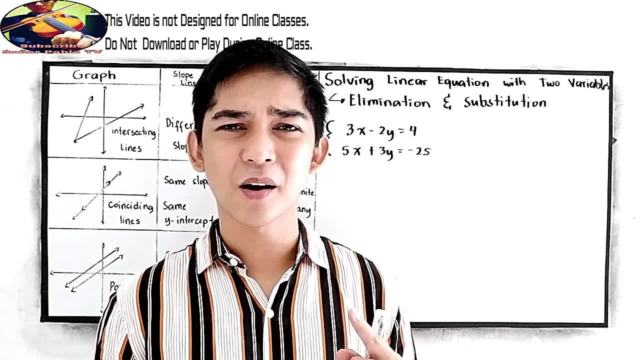 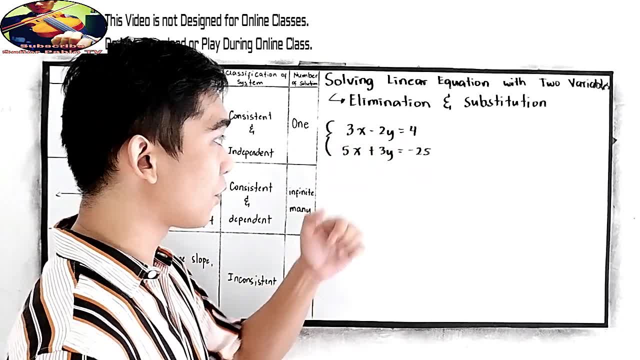 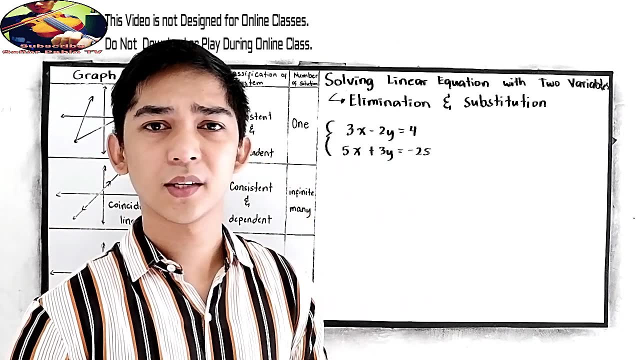 way to solve the equations. So let's try our example number one: 3x minus 2y is equal to 4 for our first equation, and 5x plus 3y is equal to negative 25 for our second equation. 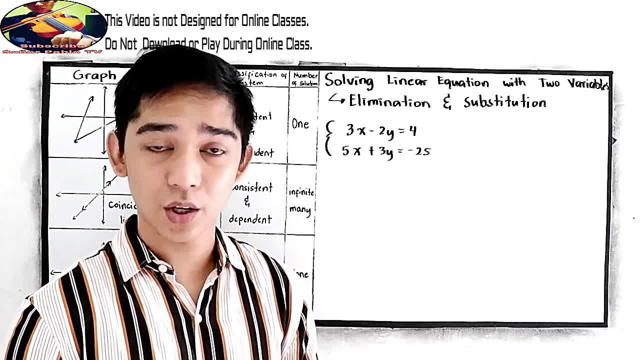 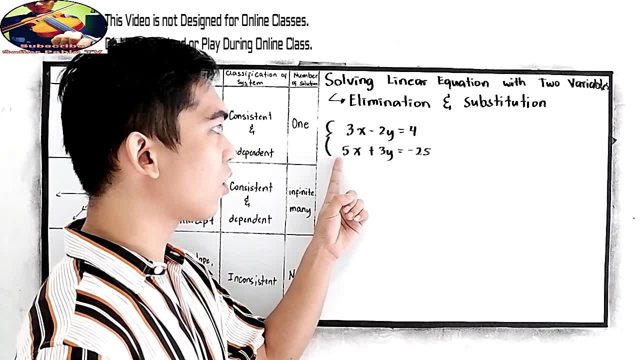 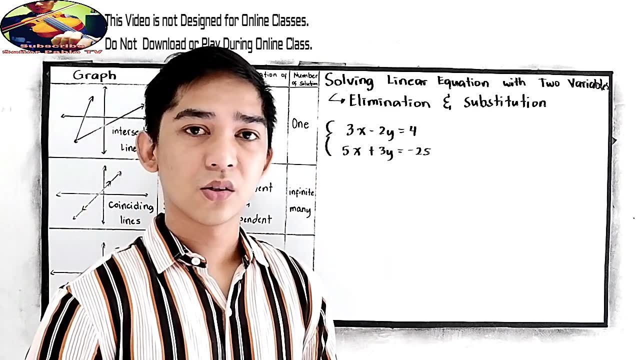 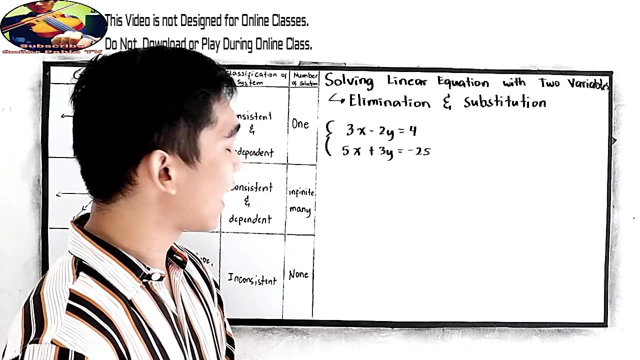 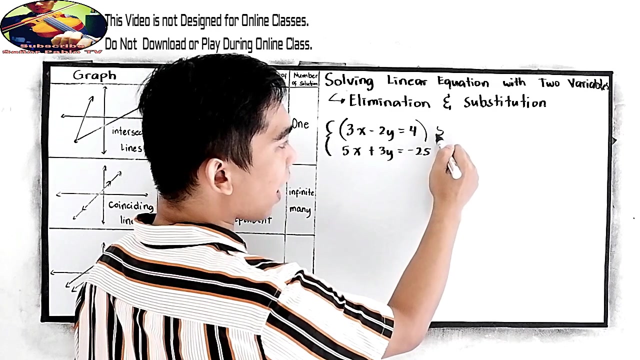 Study the given equations: For our x the coefficients are not equal, For our y the same. So if we're going to use the elimination and one elimination method and want to cancel x, so we need to cancel x, or we want to cancel x, so we need to multiply this by 5.. 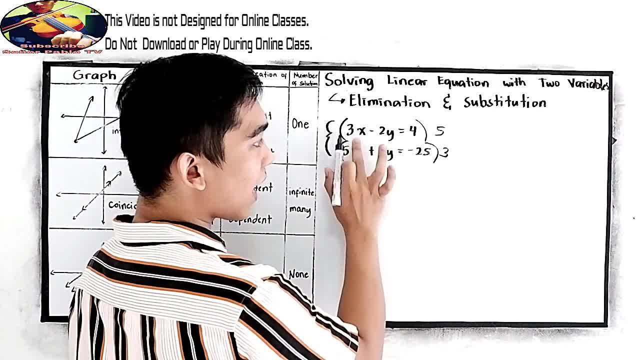 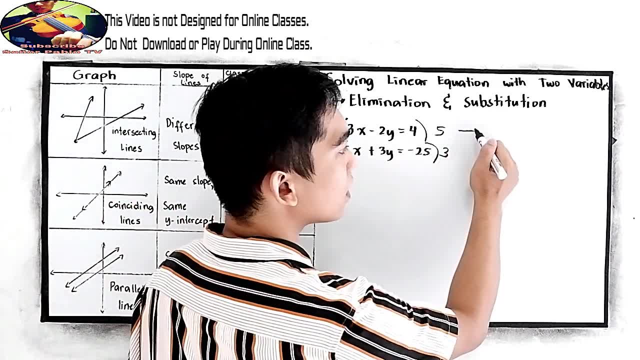 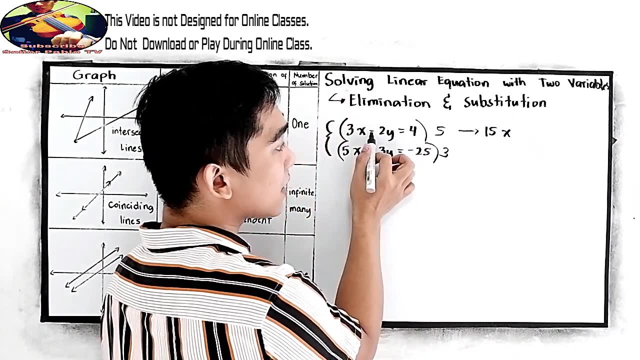 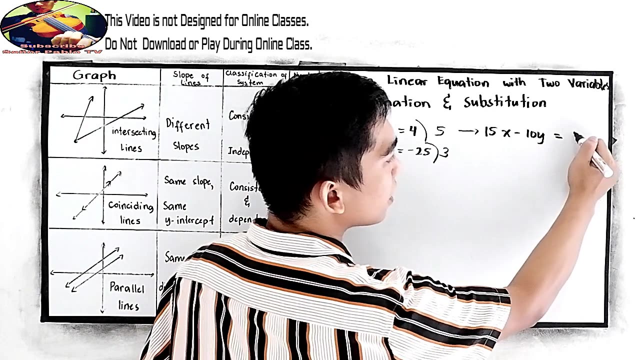 And this is by 3.. So that the coefficient for x will be 15.. Okay, let's do that. So 5 times 3x is 15x. 5 times negative, 2y, negative 10y is equal to 4 times 5, 20.. 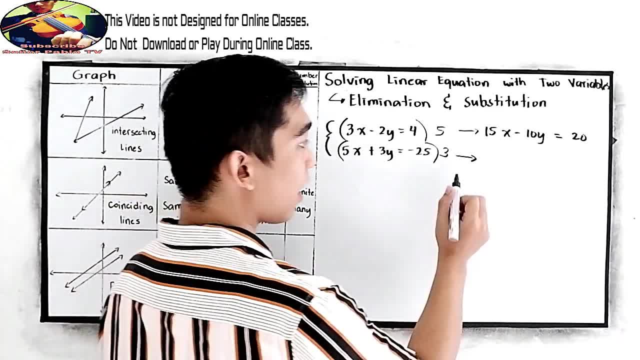 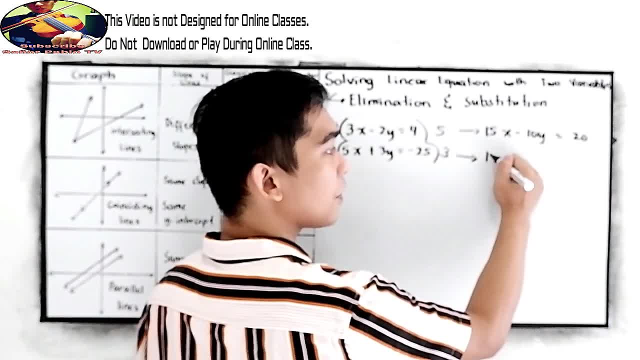 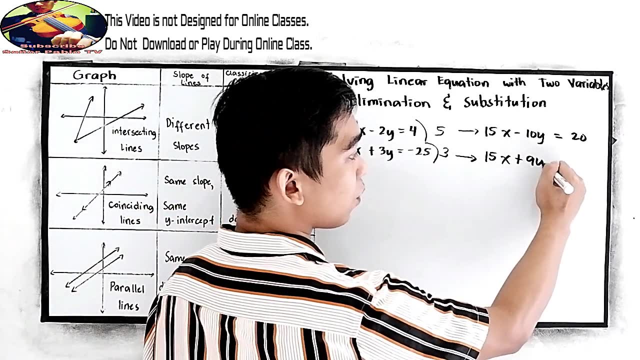 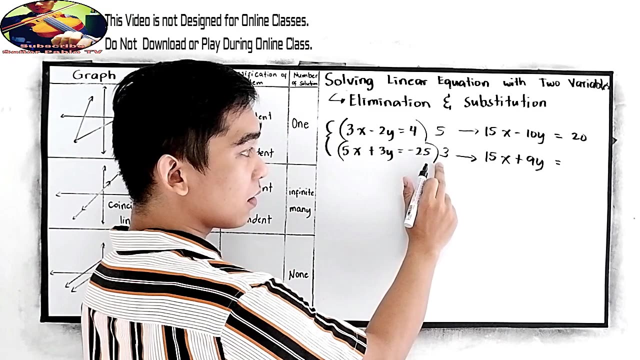 Next: 5 times 5x. 5x times 3,, sorry, 5x times 3,, that is 15x. Positive 3y times 3 is positive 9y. It's equal to negative 25 times 3,, that is negative 75.. 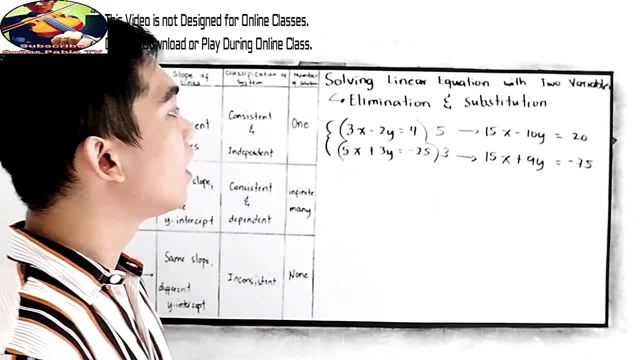 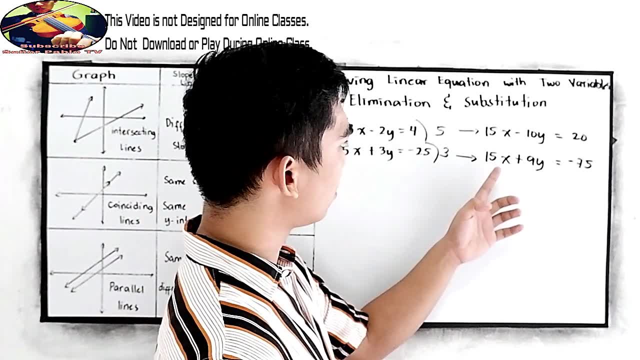 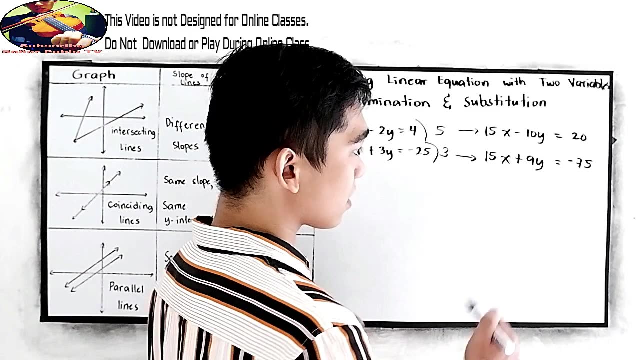 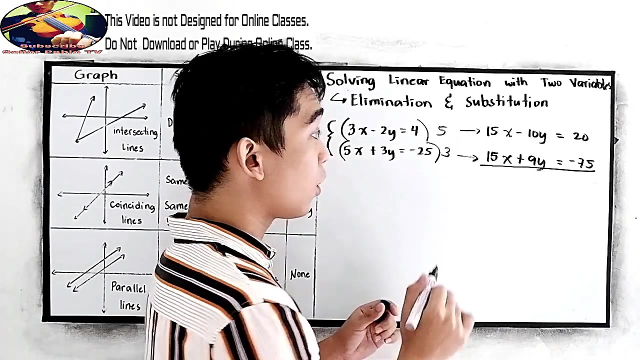 Okay, Now study the given or the equations that we produce when multiplying by 5 and 3.. So we have now the same coefficient for x. We can now cancel this. Now we're going to subtract, So 15x minus 15x will be 0. 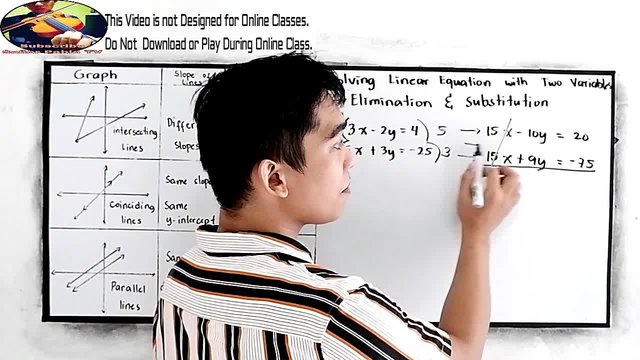 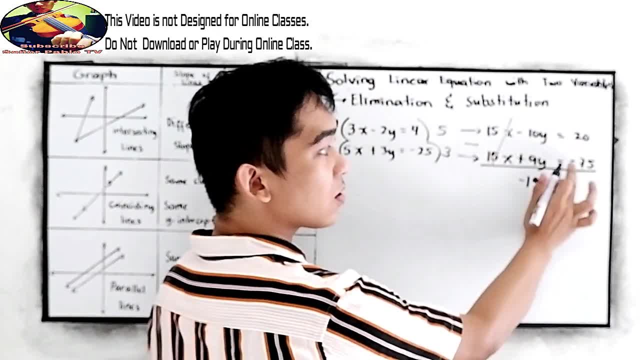 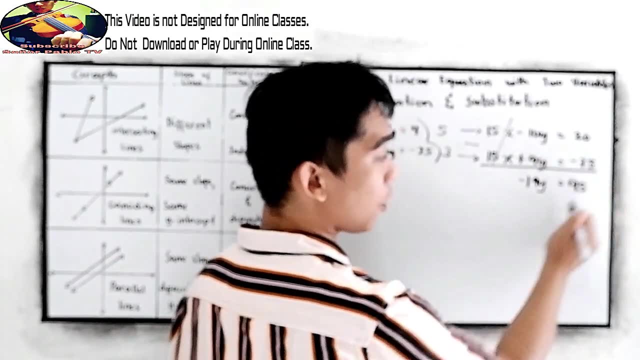 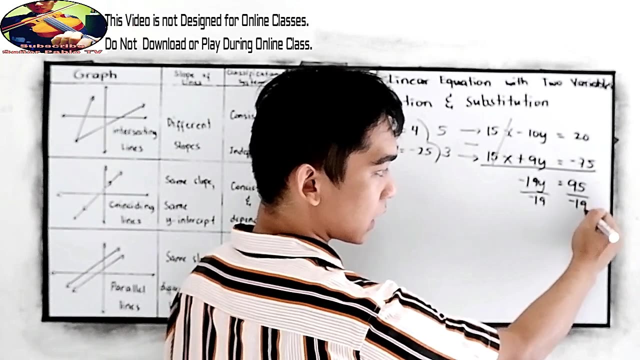 Or we can just cancel that Negative 10y minus 9y, that is negative. 19y is equal to 20 minus negative 75. So that will be 95, positive 95. Divide by negative 19. So we have: y is equal to 95 minus 9y. 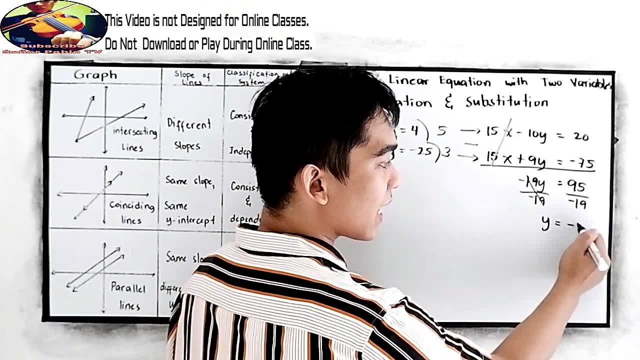 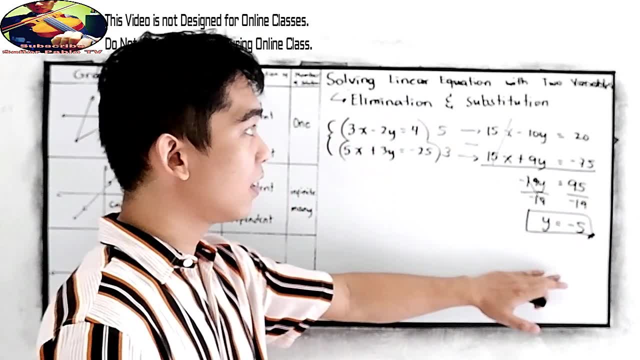 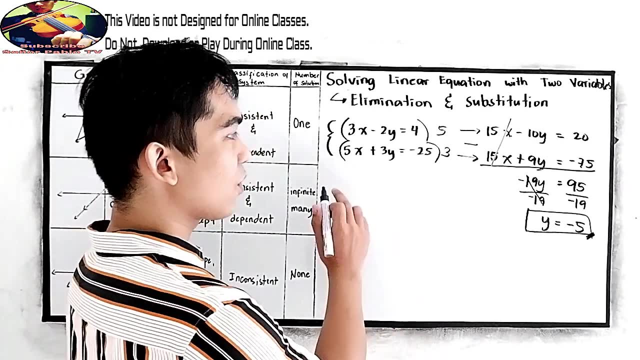 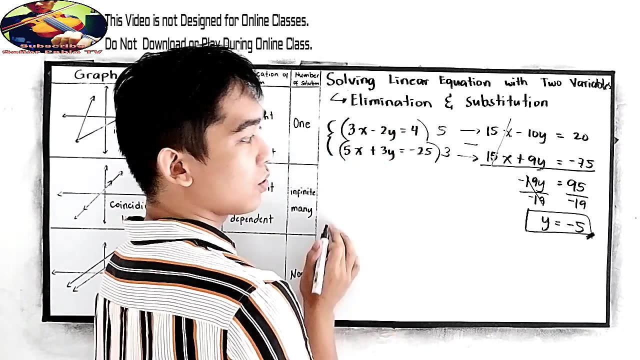 Okay, So we have negative 95 over negative 19,. that is negative 5.. Okay, After getting the value for y, let us use the substitution method to find the value for x. So copy any of our equation, So it can be equation 1 or equation 2.. 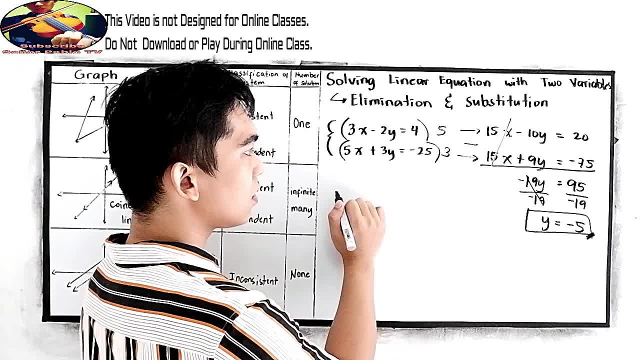 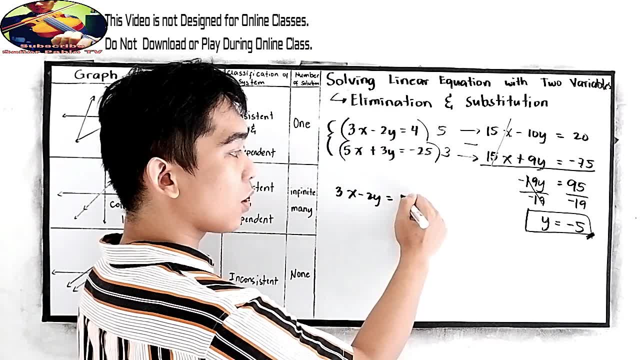 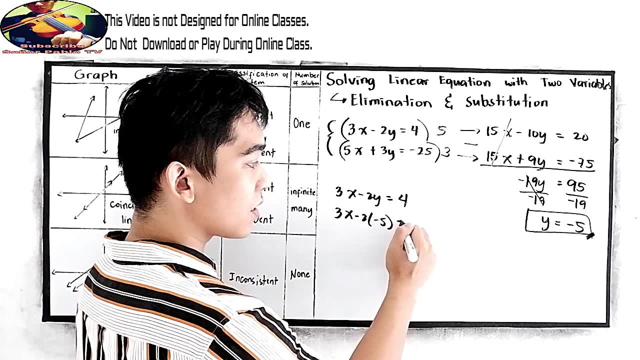 Now let us use the equation 2. Equation: 1. Equation 1. 3x minus 2y is equal to 4.. So 3x minus 2 times our y is negative. 5 is equal to 4.. 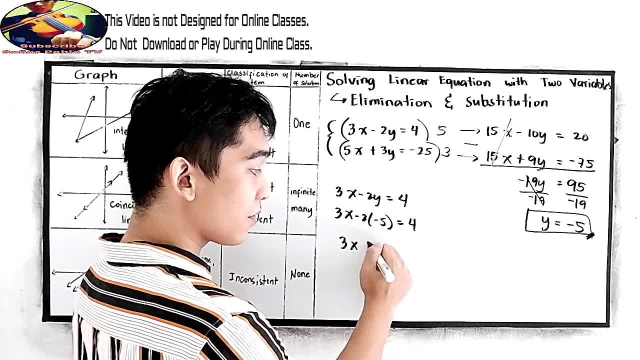 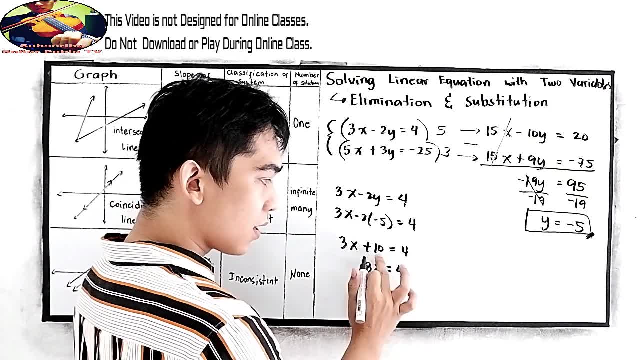 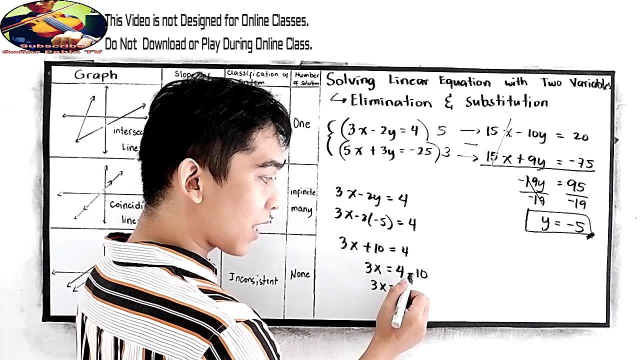 So we have 3x negative, 2 times negative. 5 is positive, 10, is equal to 4.. So 3x is equal to 4.. Addition property of equality Minus 10.. Minus 10,, so 3x is equal to 4 times negative, 10, negative, 6.. 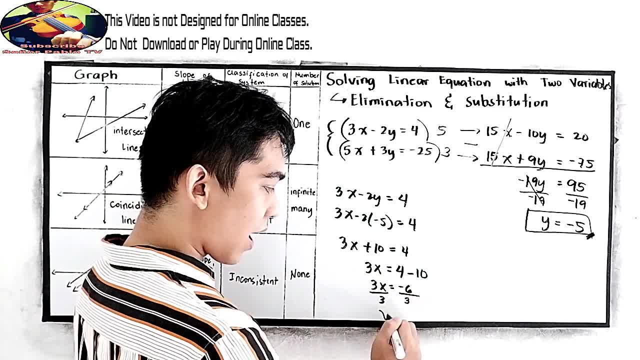 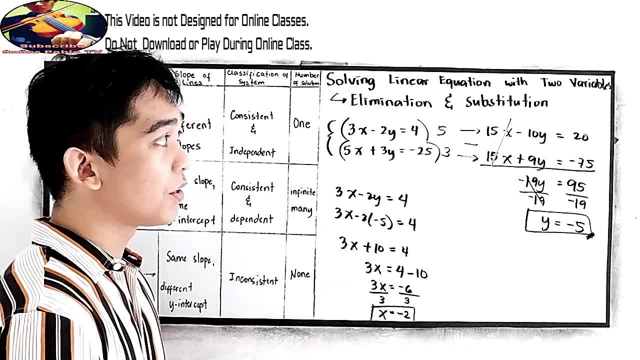 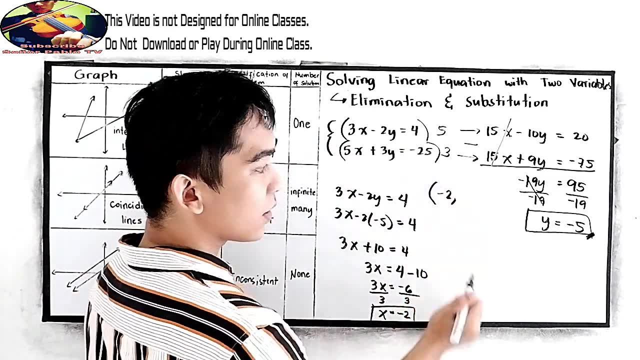 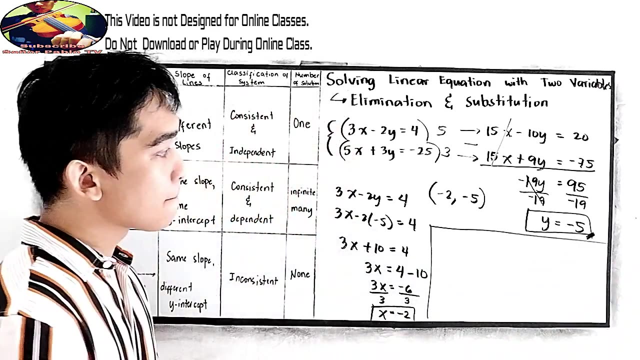 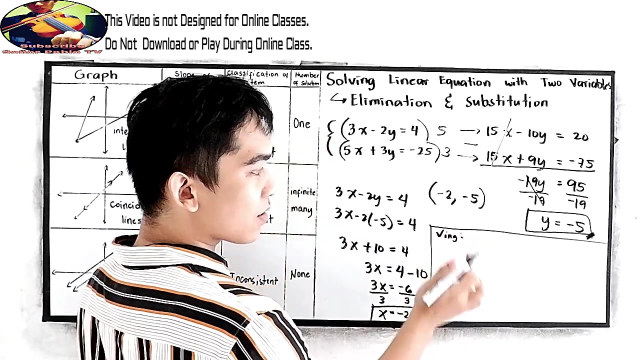 Divide both sides by 3.. X is equal to negative 3. So our x is equal to negative, 2.. Therefore, the solution of our equations are negative, 2 and negative 5.. Okay, Bye, and now let us check our answer. for the checking. this is going to substitute 3x. 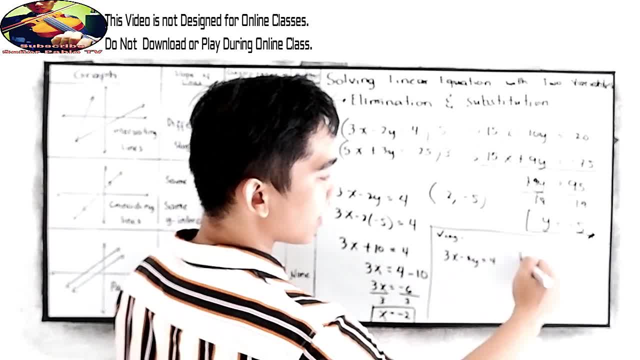 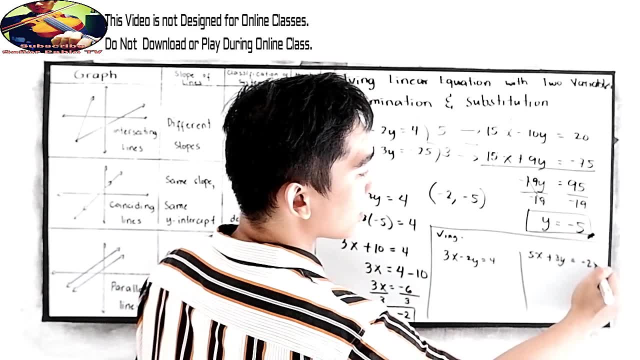 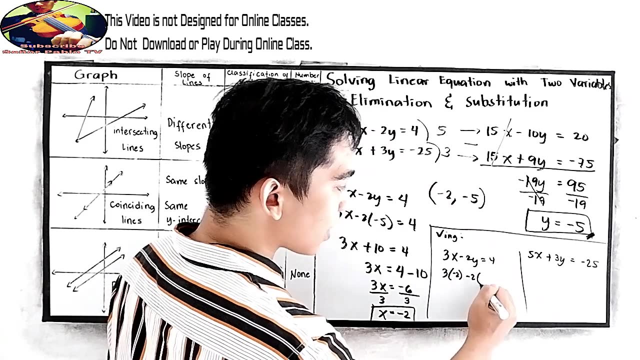 minus 2y is equal to 4 and the other one, 5x plus 3y, is equal to negative 25. so negative 2 for x. so 3 times negative 2 minus 2 times negative 5 is equal to 4. 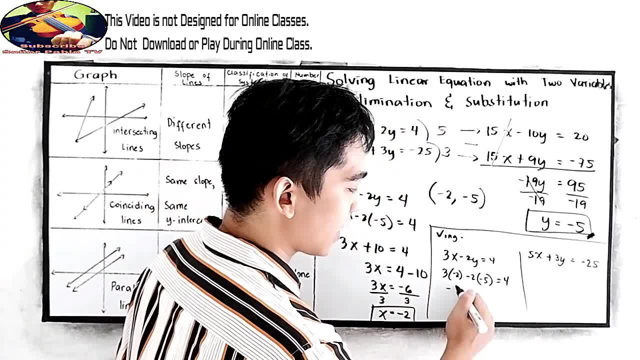 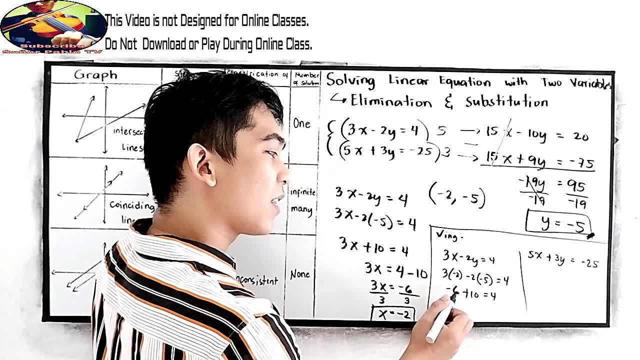 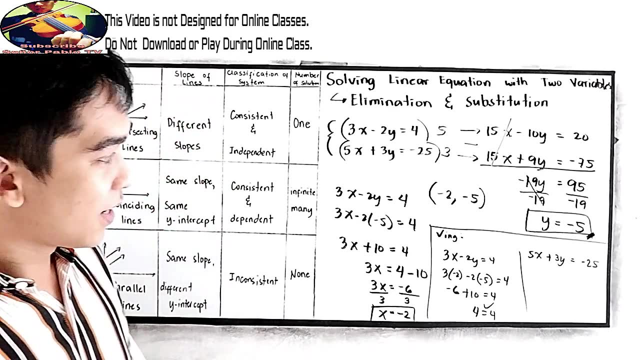 3 times negative, 2? negative, 6 negative 2 times negative, 5? positive. 10 is equal to 4, negative, 6 plus 10, that is, 4 is equal to 4, which is true, and the other one 5 times. 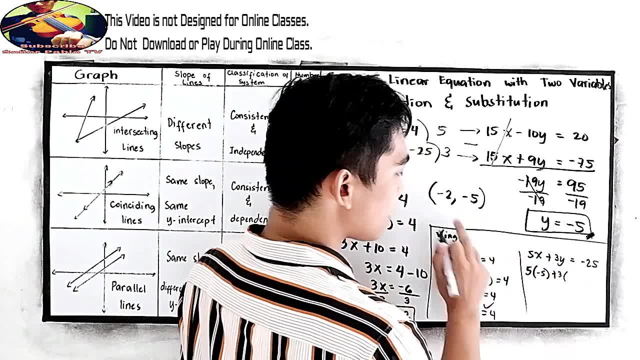 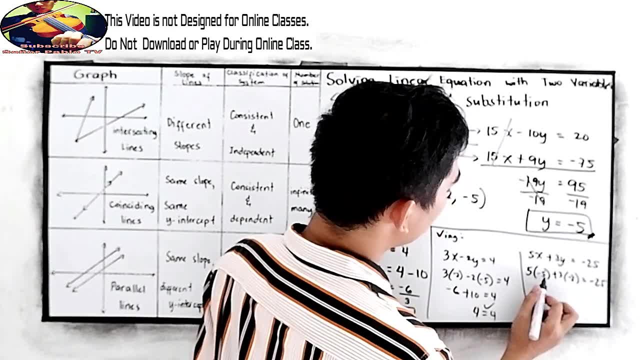 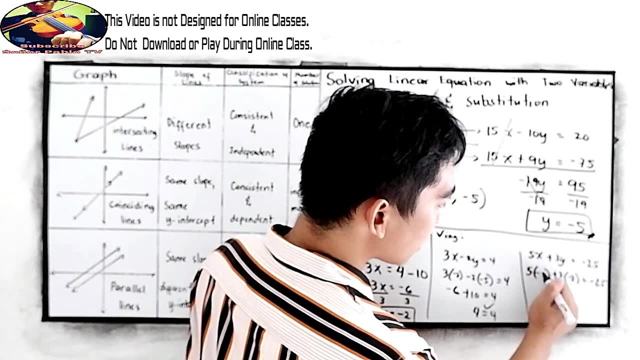 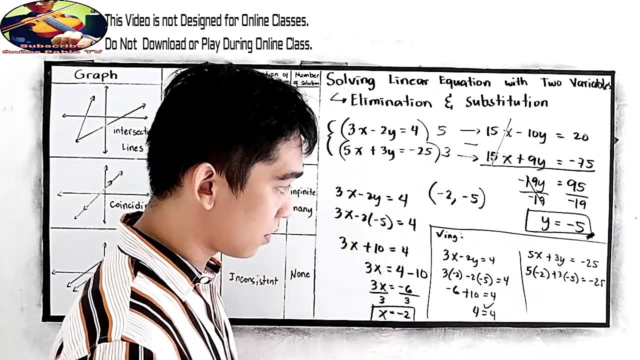 Negative. 5 plus 3 times negative 2 is equal to negative 25.. 5 times negative: our x is negative, 2. Negative 2. And our y is negative 5.. Be careful in substituting the value for the x and y. 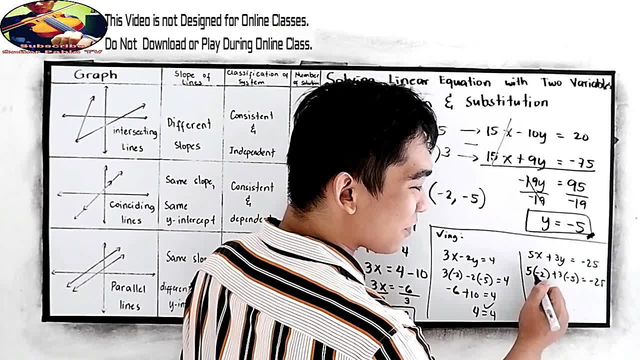 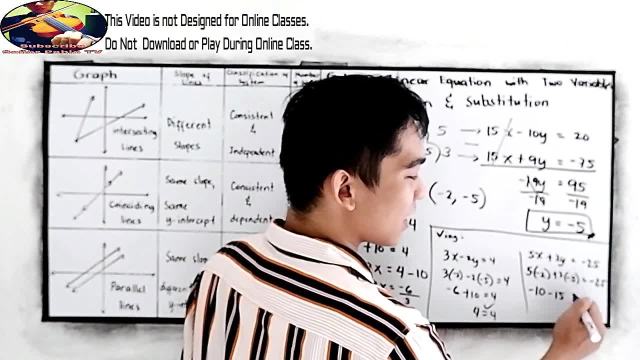 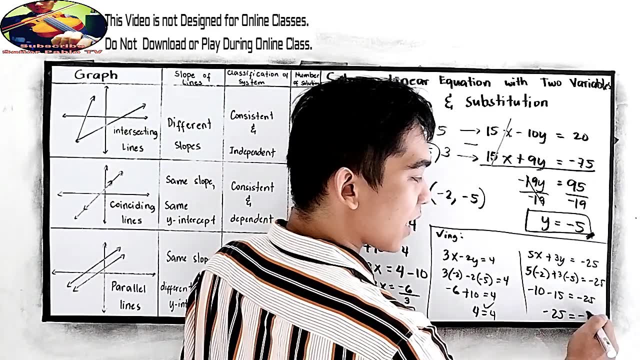 So 5 times negative: 10,, 5 times negative: 2, negative 10.. 3 times negative: 5, negative: 15 is equal to negative 25.. Negative: 10 minus 15, negative 25 is equal to negative 25.. 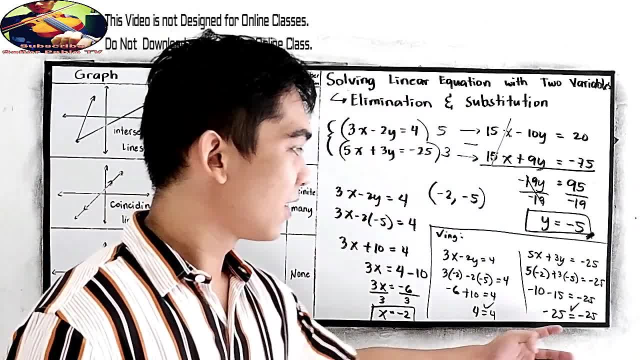 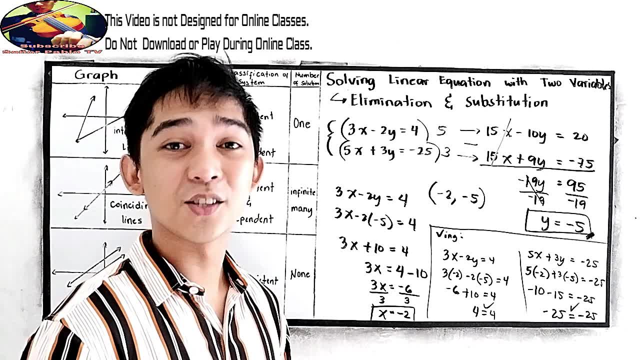 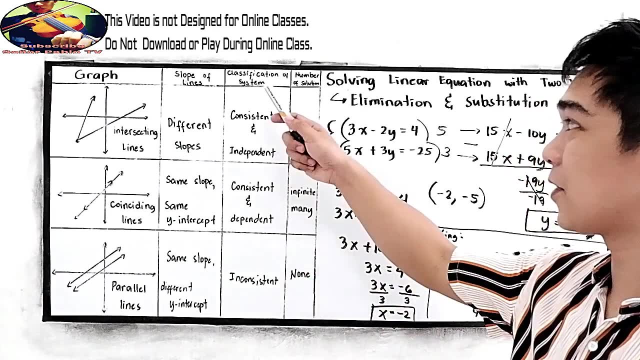 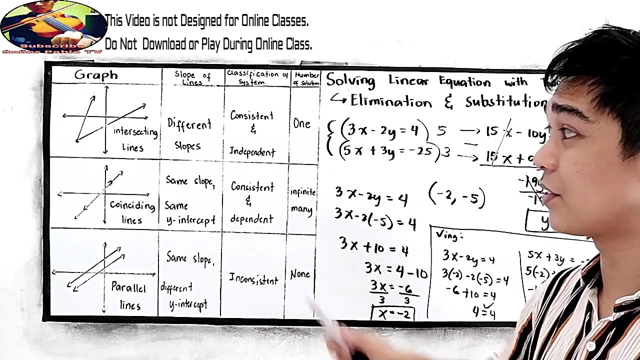 Which is also true. Therefore, our answer- negative 2, negative 5.- Is correct. Now, if your teacher or the person asks you: what is the classification of the system? So consistent and independent? We have the number of solutions: 1 and the intersecting line. 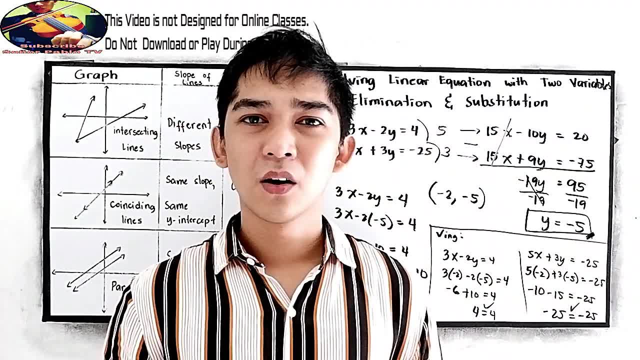 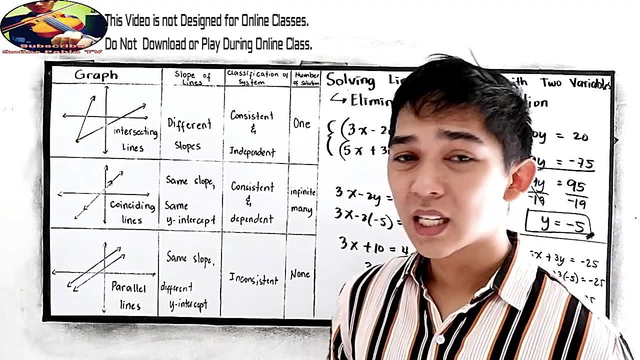 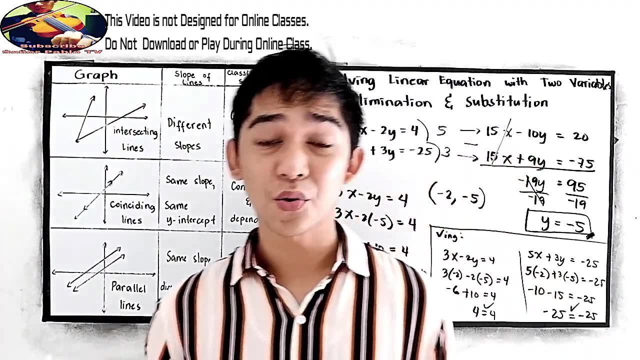 Now in our next video. What if you're going to find out that the equation, or the system of equation, Is a constant and parallel line? So we haven't encountered that, So that would be our next lesson. What will happen if that would be the graph? 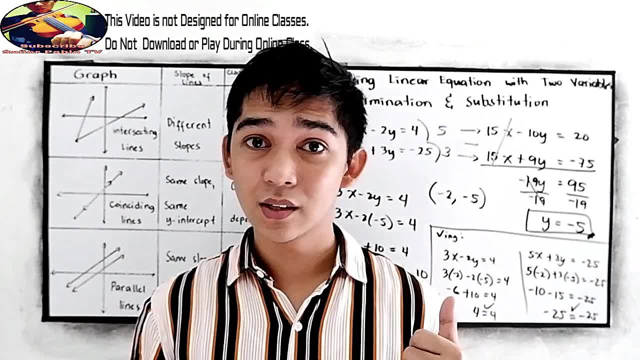 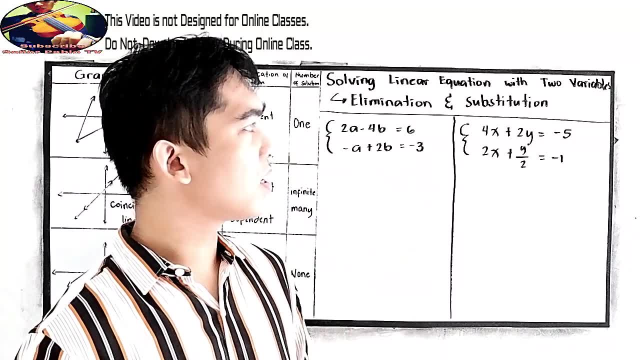 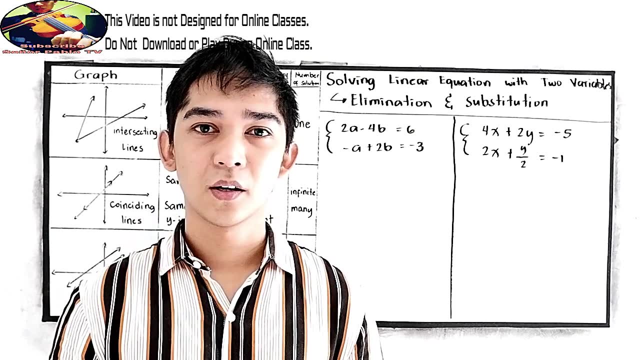 So stay tuned for the next video. See you in our next examiners. Thank you for watching senior public. The system of linear equations with two variables, using the substitution or the elimination. But put in mind We're going to use the substitution or the elimination. 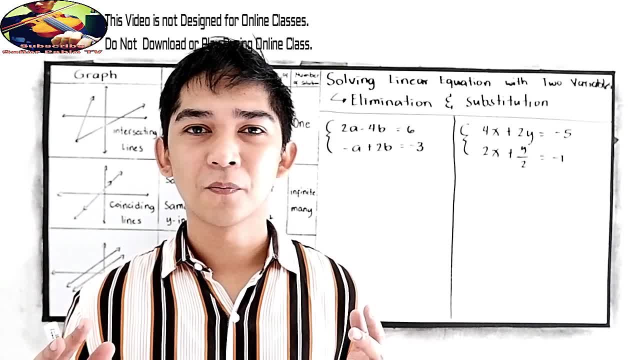 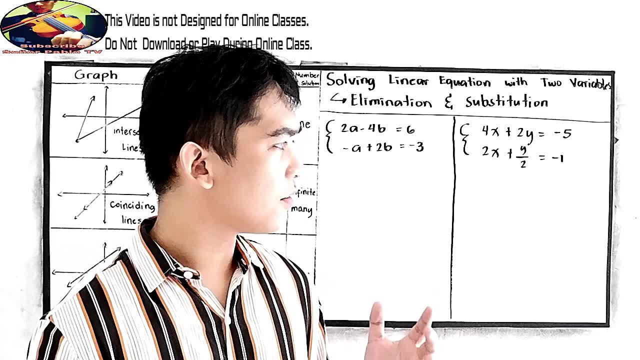 But put in mind We're going to use the substitution or the elimination. But put in mind We're going to use the substitution or the elimination. So if we're going to find The value for our X&Y, But notice the given. 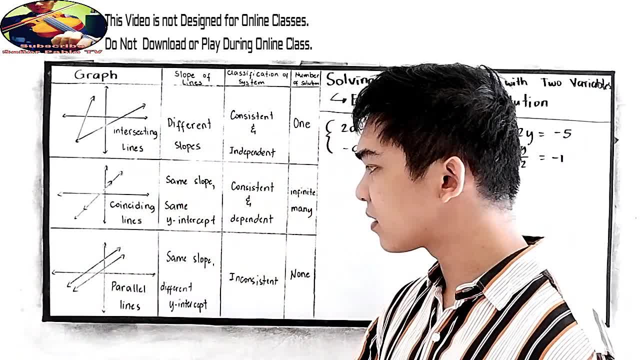 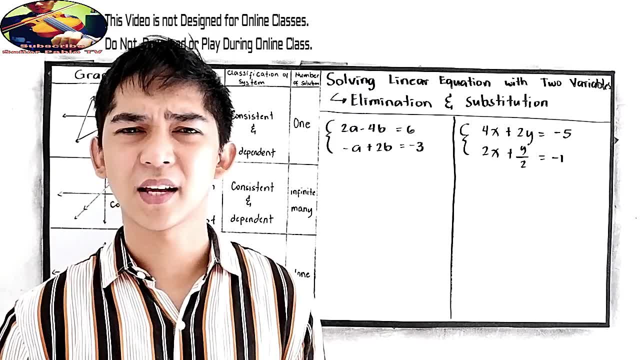 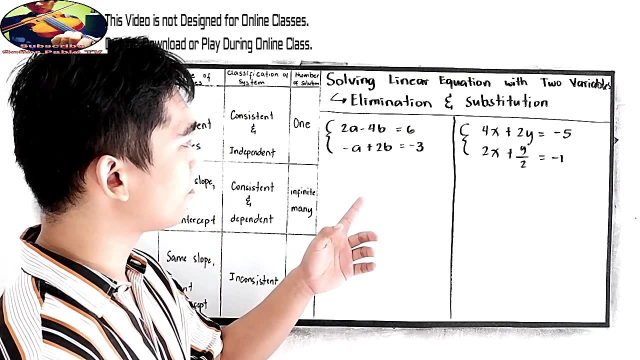 That we will come up with the coinciding lines and parallel lines. So if we're going to graph that, That would give us the coinciding and parallel lines. So what will happen to our X&Y? So let's try this example number 1.. 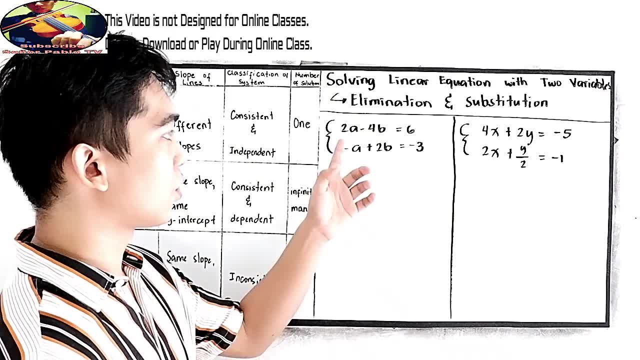 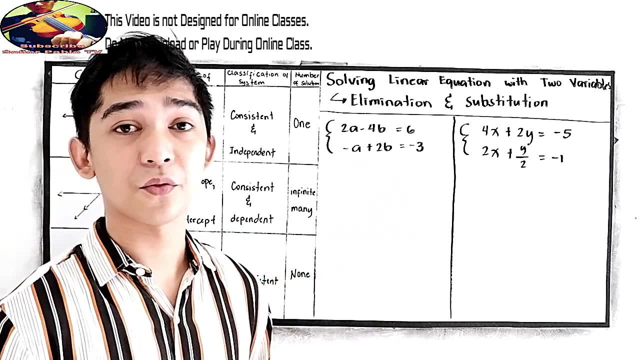 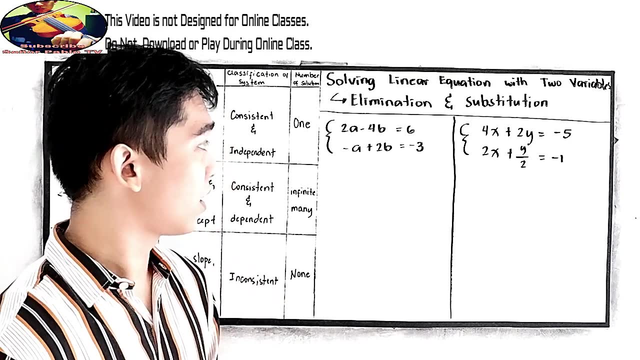 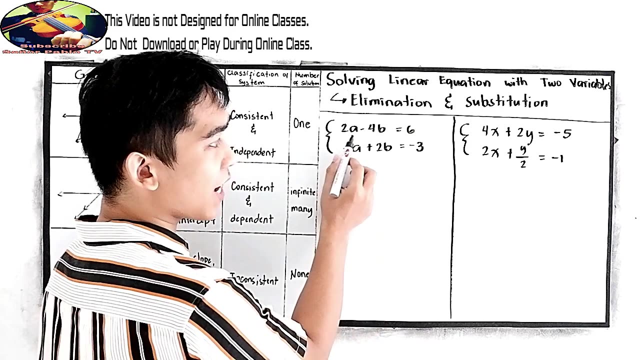 So 2x minus 4b is equal to 6 and negative a plus 2b is equal to negative 3.. So we're going to use the elimination method, the easiest way to solve this. So our goal is the coefficient for a in both equation one and equation two must be the 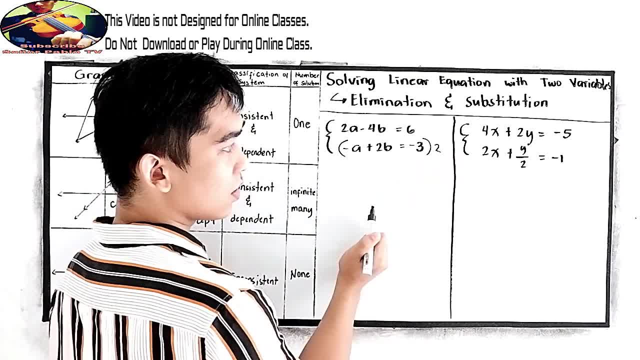 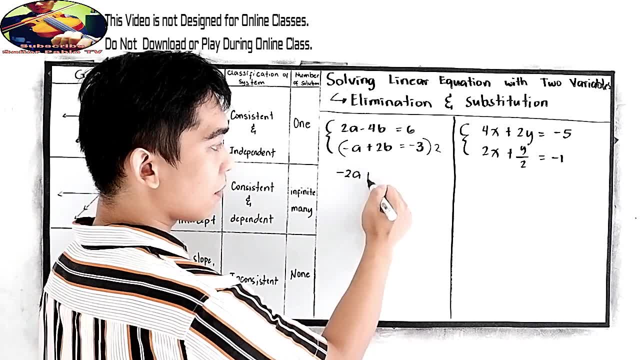 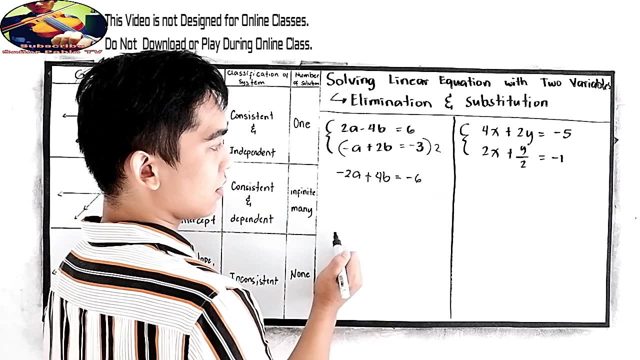 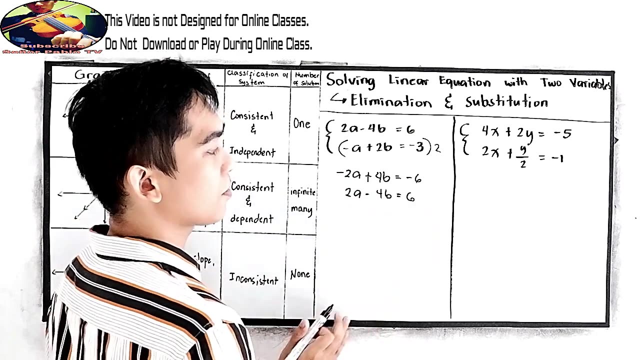 same. So all I need to do is to multiply two in our equation two so that it will become negative. 2a plus 2 times 2b, 4b is equal to negative. 3 times 2, negative 6.. And just copy the equation one: 2a minus 4b is equal to 6.. 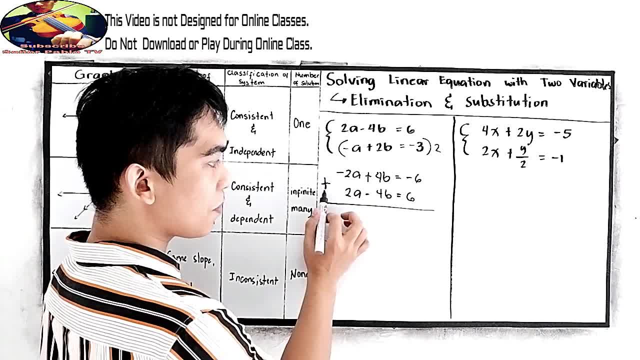 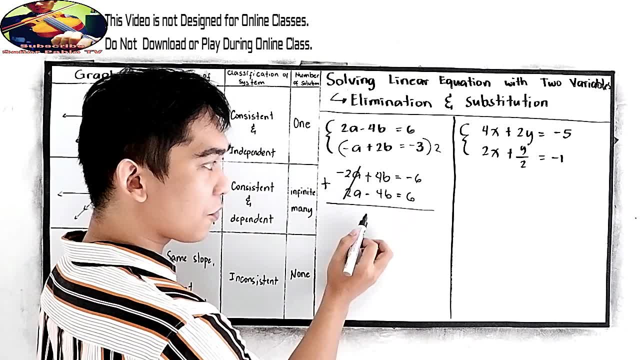 We're going to add, So we're going to add, So we're going to add, So we're going to add 2a plus negative, 2a plus 2a. this is zero. Four plus negative four, this is also zero. 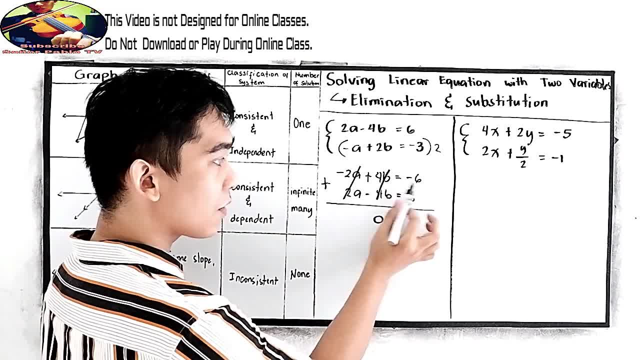 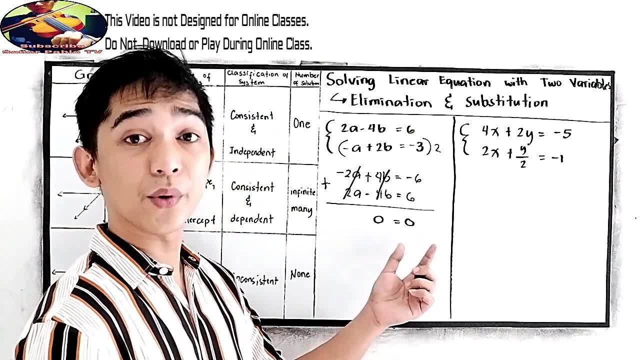 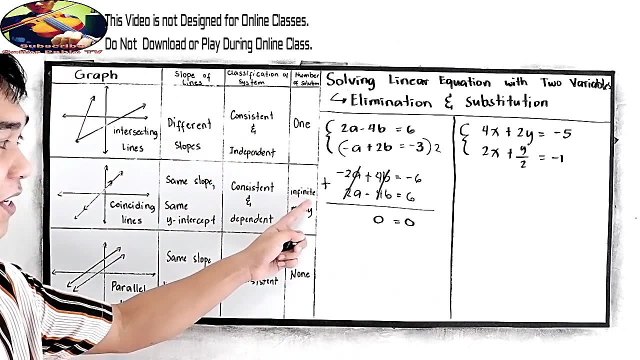 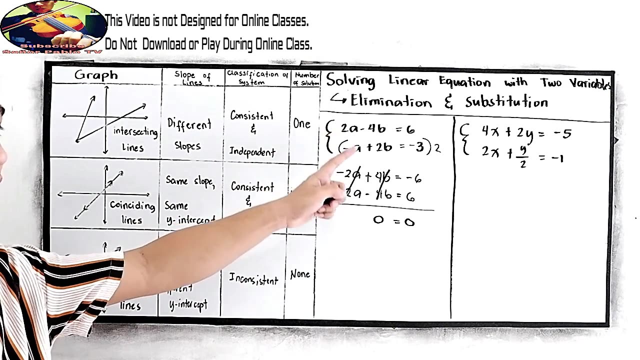 So zero is equal to negative. six plus six. this will also give us zero. So our equation will give us: zero is equal to zero. So that gives us the infinite many solutions. If we're going to graph the two, the equation one and the equation two, this will be our. 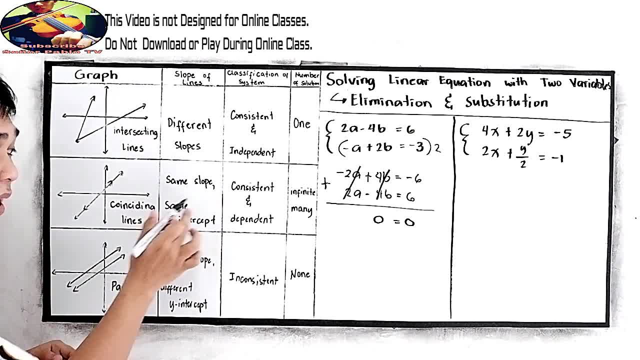 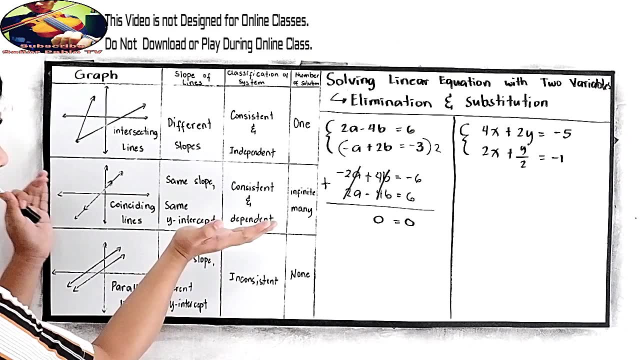 graph. So they have the same slope and the same y-intercept And for the classification of system, consistent and dependent. Okay, Now it's clear to you what it looks like if we're going to solve our equations. the coinciding lines: 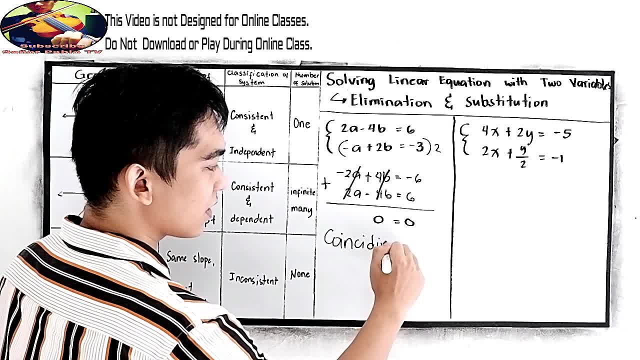 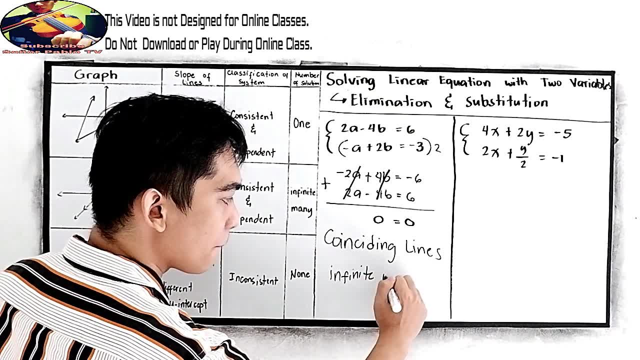 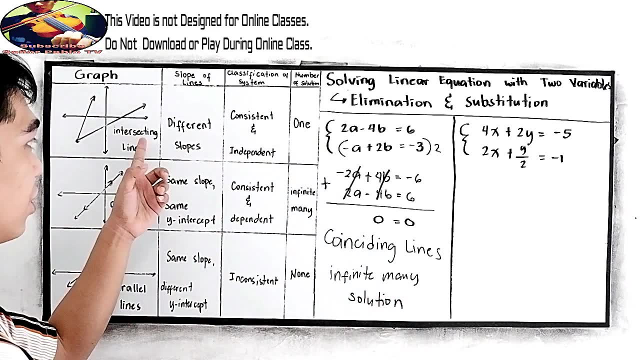 Okay, This will give us coinciding lines, Infinite many- solution, Unlike our unique solution or the intersecting line. we're going to graph that and we're going to be at exactly one point In this case. why infinite many? Because our points is infinite. 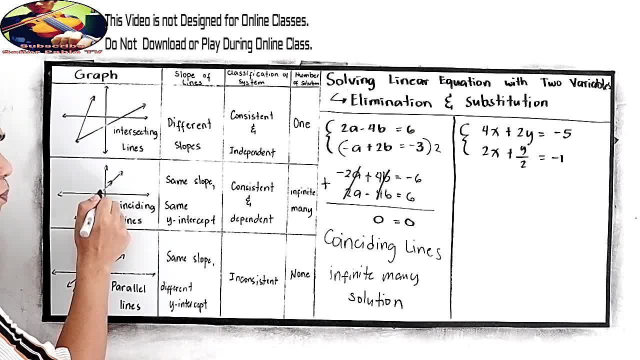 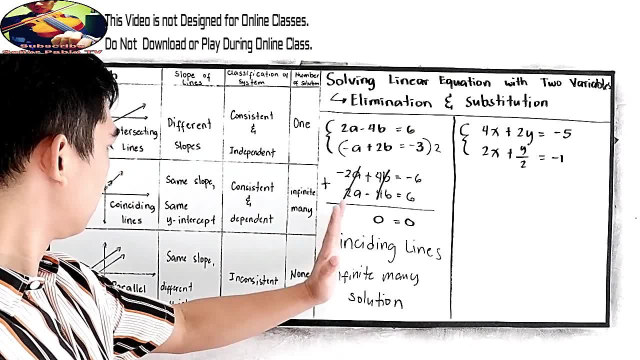 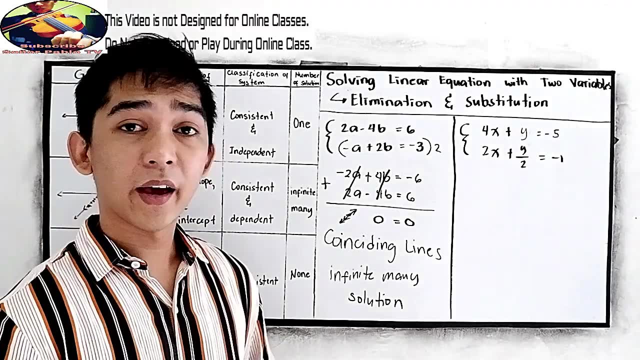 There's a lot. A line is composed of infinite many points. Okay, So that's the coinciding line. So our graph will be like this one. And now let's try our example number two: Four x plus y is equal to negative five. 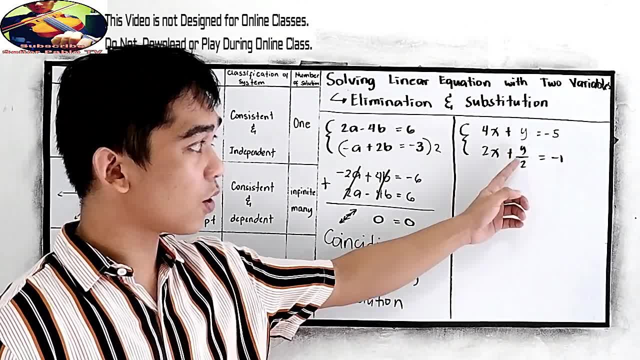 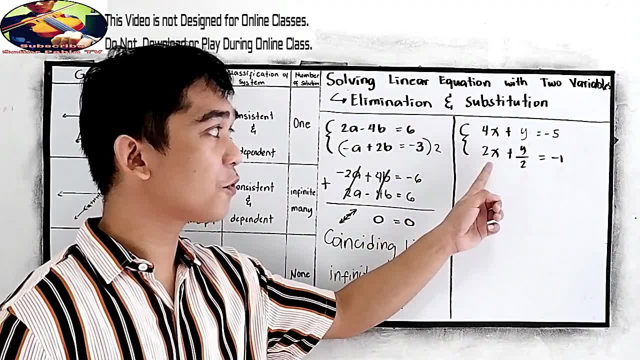 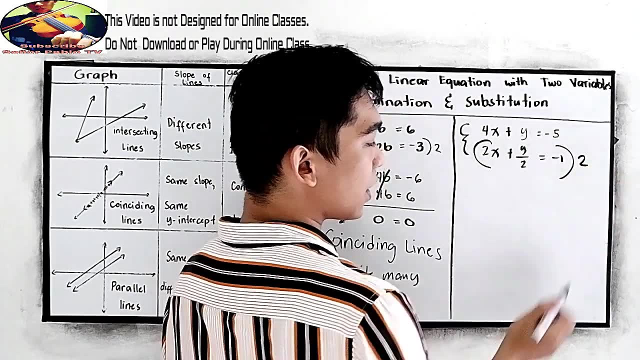 And the equation two is two. x plus y over two is equal to negative one. Using the elimination method. Using the elimination method, our coefficient for x must be the same, So all we need to do is to multiply two in our equation number two. 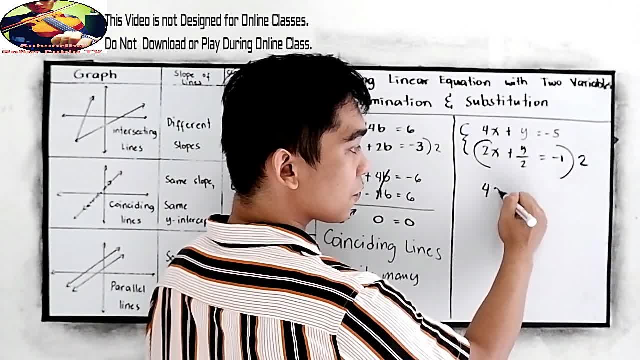 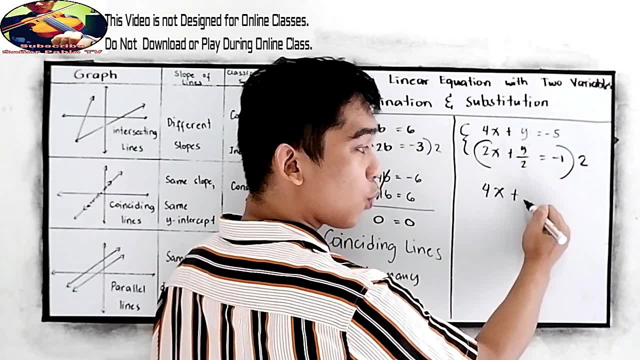 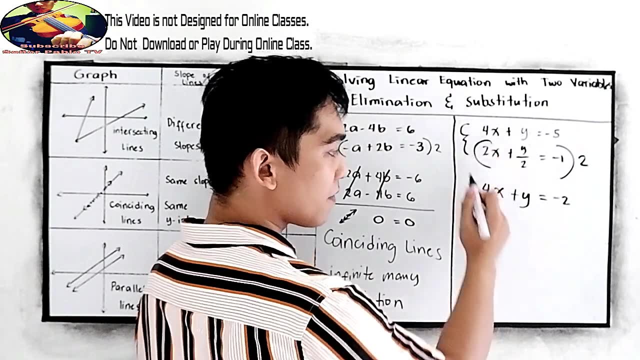 So two x times two gives us four x. So two divided by two, that is one times y, that is one y, or simply y is equal to negative one times two, negative two. Now four x plus y is equal to negative five. 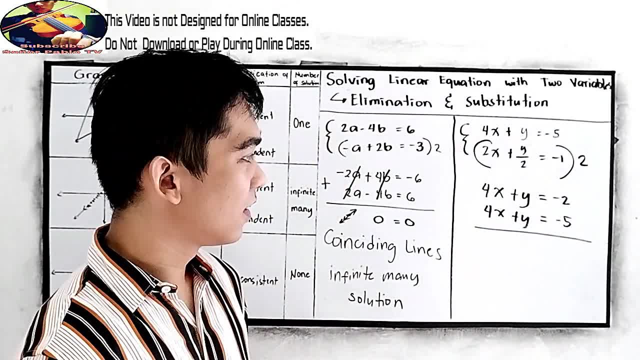 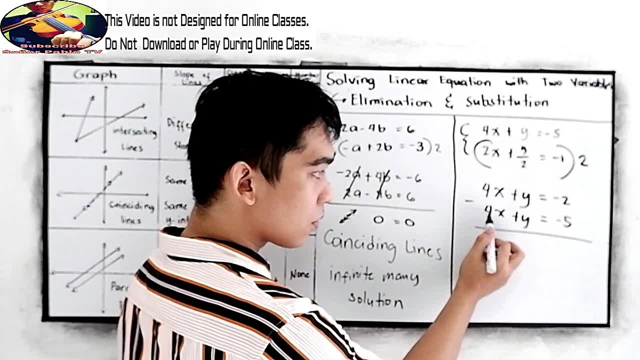 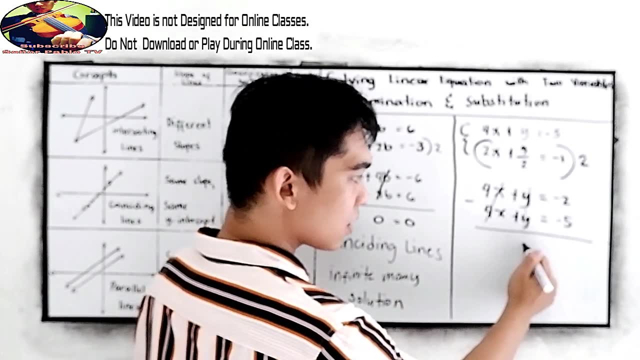 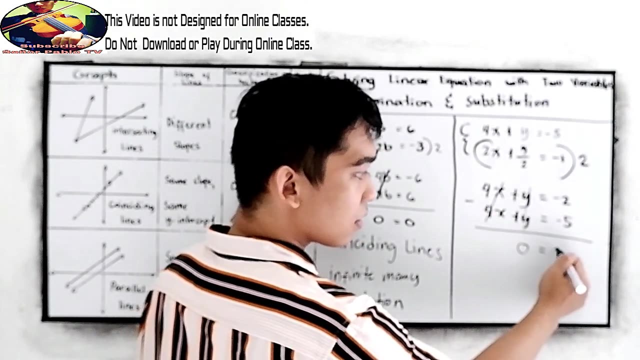 Just copy the equation one And let us subtract Four x minus four x, that is zero. Y minus y is also zero. So this gives us zero is equal to negative. two minus zero Plus negative five positive three, So zero is equal to a number. 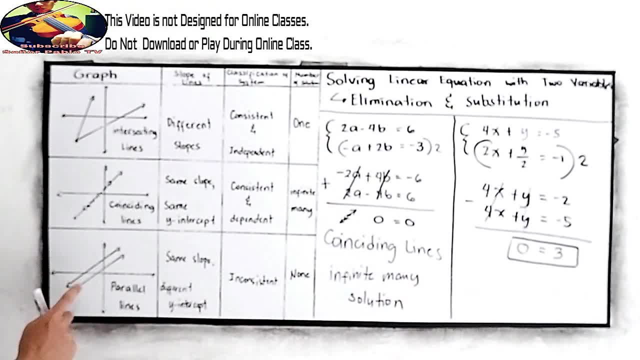 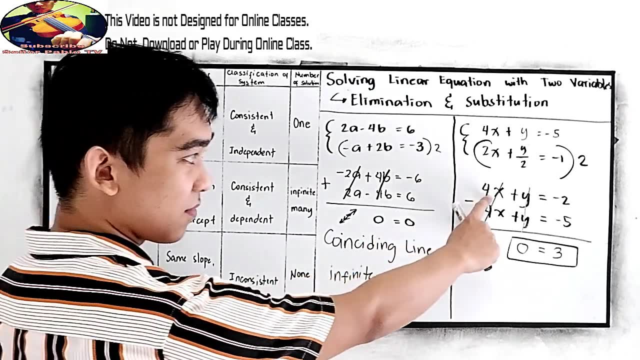 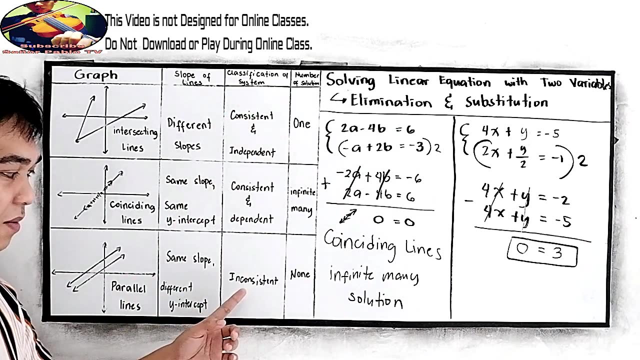 So we're going to graph. This will give us the parallel lines. Notice that they have the same slope but different y intercept. Their slope is negative four And the classification of the system is inconsistent And the number of solutions there is none. 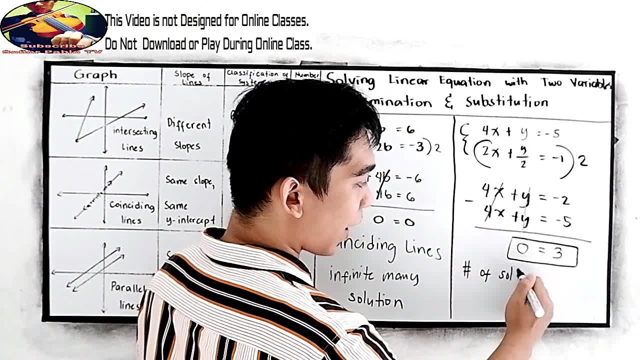 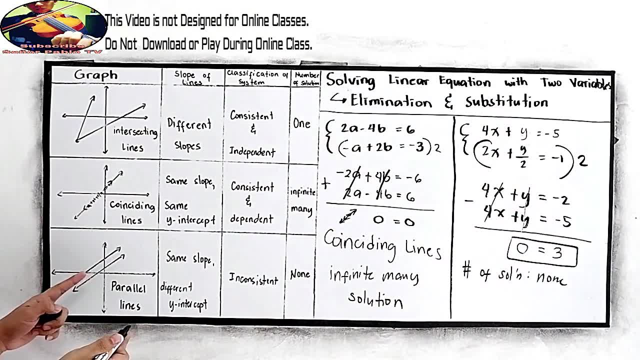 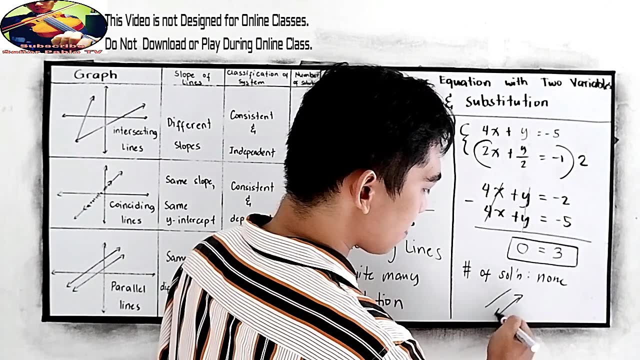 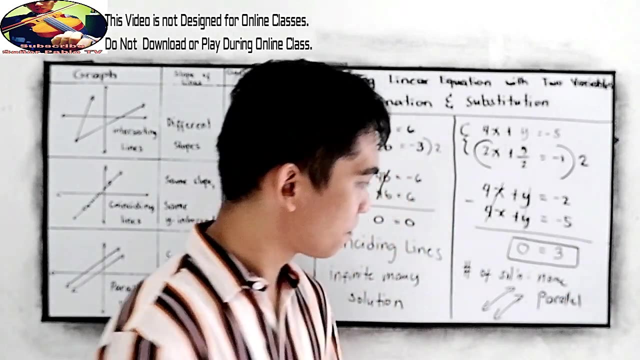 Number of solutions: none. Why none? Because our two lines will never meet at any point. Of course, in our graph we're going to graph. in our partition plane The two lines are parallel. Okay, So you can easily find those in our solving linear equations. 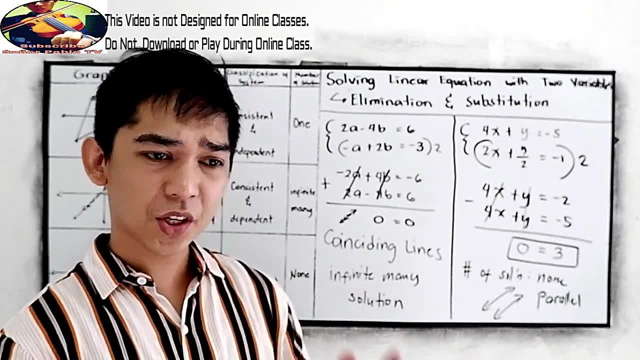 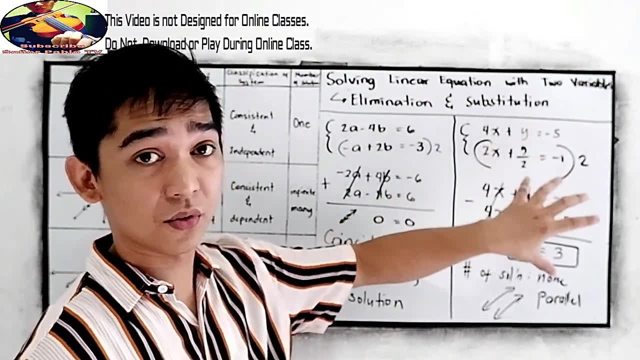 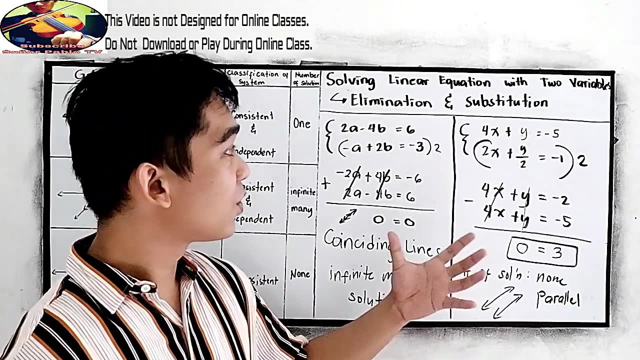 You don't need to. If your teacher asks you what is the classification of the system or the number of systems, you just need to solve. You don't need for you to graph or something like that. That's the importance of knowing how to solve the linear equations with your variables.